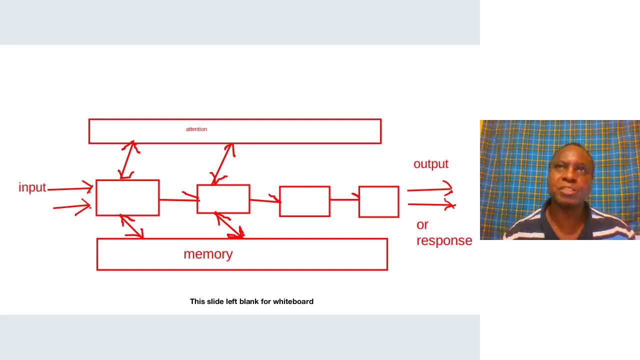 also a little more practical. suppose somebody told you their name, you meet with them the first time and they say i'm so and so, uh, so that comes through the sense of hearing. of course you have also seen them. of course, in this case, of there is also a sense of hearing, of course. 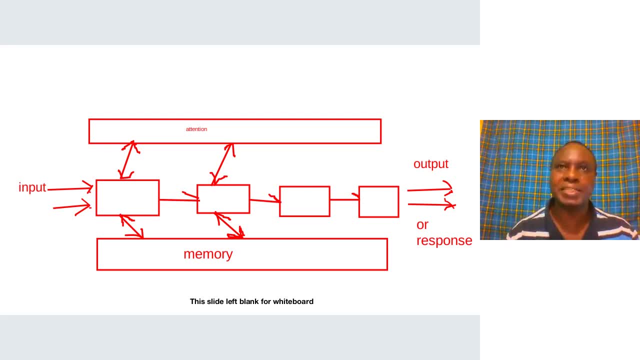 the site. so of course, we can say, is that that combination, you have seen the person, but also the person has also, uh, told, told you their name, um, so there are two things that you need to later remember. in this case you need to remember the, this person, physically, you know, if you see them. 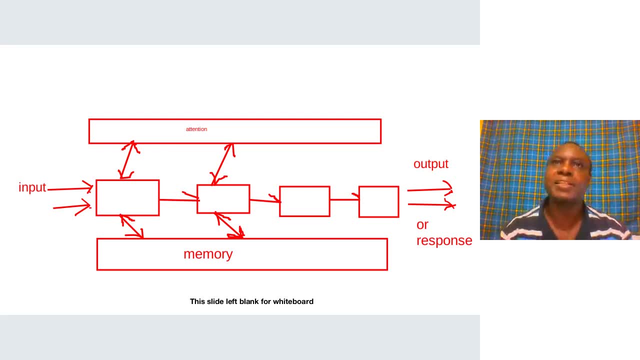 that uh say, oh, i have seen this person. but there is also now the issue of the name, so you can you also remember their name. but that's what we are saying. this said, the input comes through the senses, and the input, of course, is a whatever you have um interacted with uh through the senses, either by 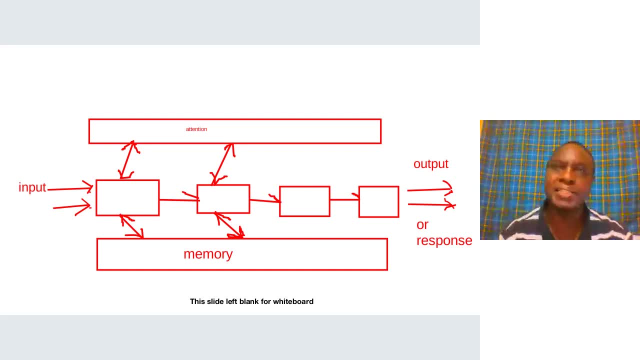 hearing, or by seeing, or by tasting, or by the sense of touch. we have the, the sense of touch, uh and uh of smell. so whatever you interact with through the senses, that, what we were interacting with the first, the time that it comes to the first time to it comes to you through that, then you 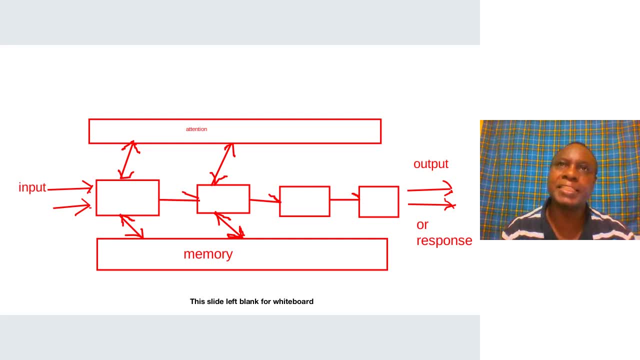 are getting the input and then it is being processed so that you have interacted with the first time- you are now or just when you are experiencing it. at that time, then it enters into the processor- in this case is a human processor. of course, at this point we don't want to get into. 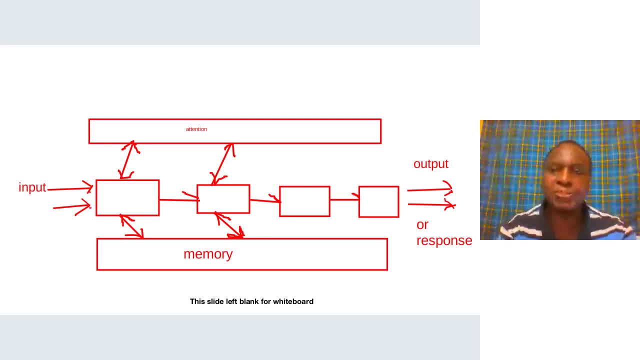 the details, which part of the human is doing the processing? but of course a lot of it has to do with the memory, i mean the brain. all right, so then it is therefore goes through there the processing, and we are saying that, as it goes through the processing, then you can. now there is a output. 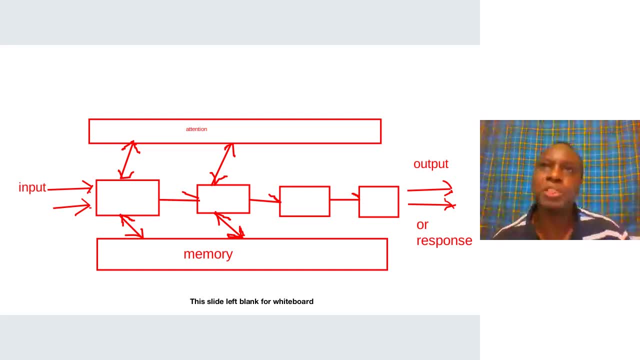 the output is: either you have gained some knowledge which you will go to the memory or you actually need to respond physically, depending on the situation. for example, of course, what? what happens if you? of course, i have not done this myself, but i cannot just imagine because i have never. 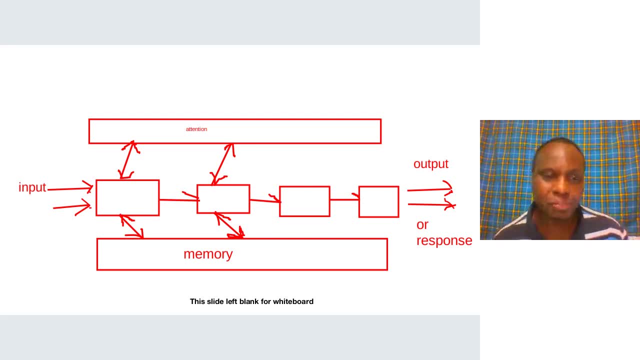 had that experience, that suppose you just all of a sudden saw a lion. you know me, you know just so. how do you react to that? now, that is going to how you react to. that is going to be the output, right, but what, uh, the the input is seeing the lion, uh, and then, of course, that goes with the. 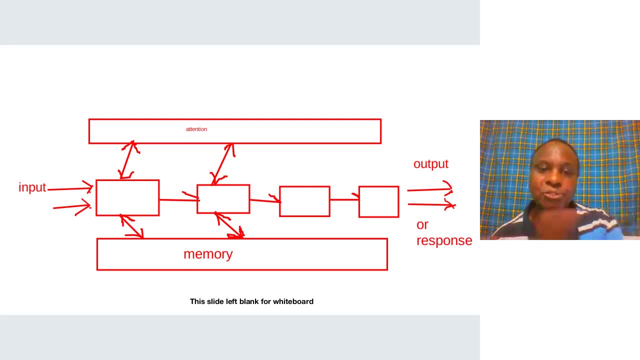 processing in some way, and then how you are going to respond to. that is what we are calling the output. how so? how do we respond? of course, there are some things that we do that become so going a l lonesome, so output. so how do we respond? of course, there are some things that we do in 블�ج� вс6. 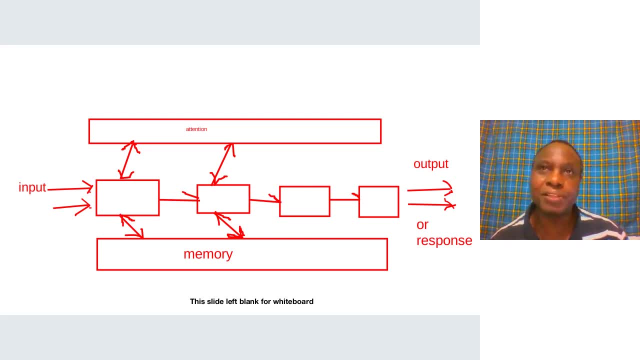 of course, one of the things that you start thinking about is a running away, but anyway, that could be one uh or hide some. maybe you are in a place where you are able to quickly uh, get into some protection and you, of course, get into that. that's a response, a physical. 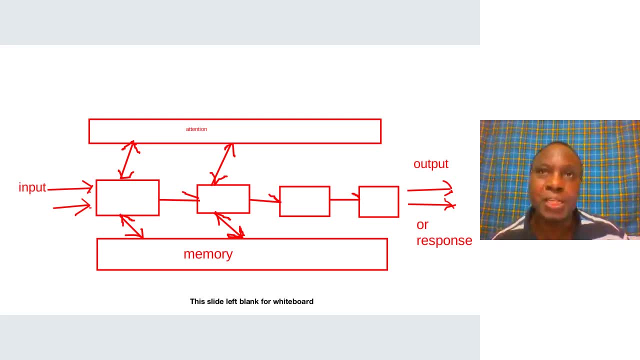 response, but there could be some other responses that are not necessarily physical, of course. one of them is: you have, you get filled with fear. uh, certainly you'll get that. there's a sense of fear, which is also an output. yes, you see the land, you get fearful about the situation. that's a, that's an. 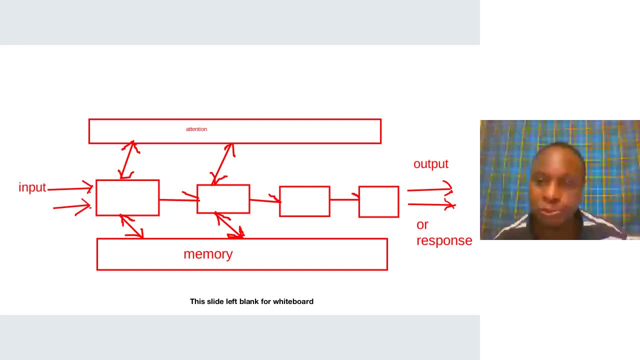 output. uh, so we, what we we're saying is that just the ordinary way we interact, we interact with the environment, that is the information, that's what we are calling the information which is being processed. so, like, as i've said, i'm trying to give the analogy of seeing a lion. so you see a lion and 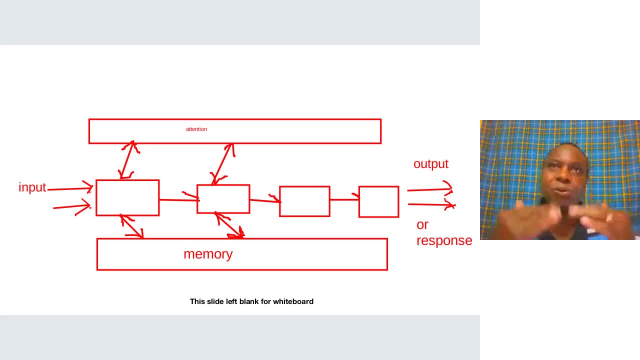 so the whole of that experience starts getting processed by your information processor. the human information processor within you starts to process that, and so, finally, you, you need to to. that is what you, what you have experienced, is, of course, going to bring out an output of some sort. 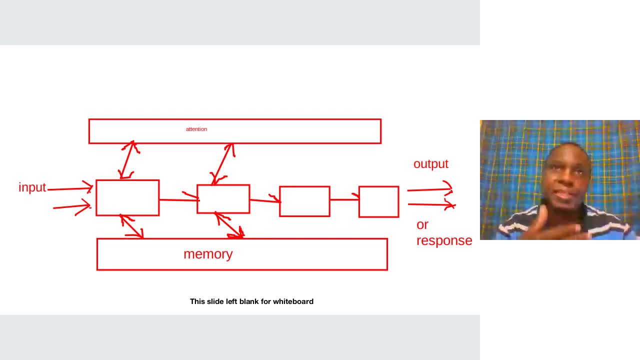 and i said maybe one of them would be: you are filled with fear, otherwise, well, you did not have fear before, so something is happening. uh, so you have the fear. you not now, of course. then, quickly, that fear may also guide to do further. responding as an output. 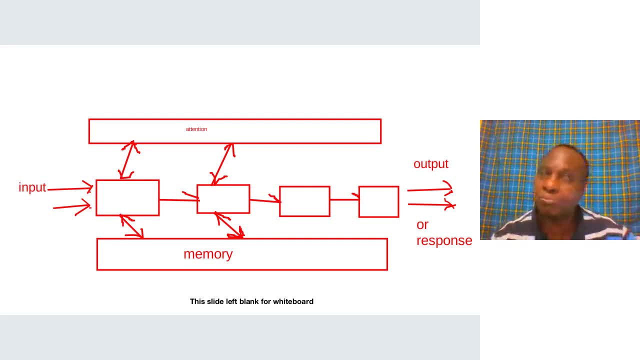 maybe to. if you think that you can run as fast as you can, then you run. or if you are near some place you can get some protection, then you run quickly into the protection and maybe hide yourself. all these are part of the output, the output of what you have experienced at that point. 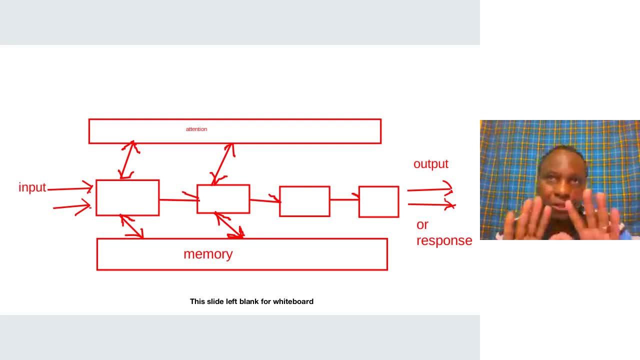 and so the when you first see the lion, that is the other, the input: you have seen a lamb, and then, so that is of course. this, of course, should be very fast. some of these things, uh, happen very fast. uh, the processing, of course, is not something that's going to take, you know, a long, long time. it is a. 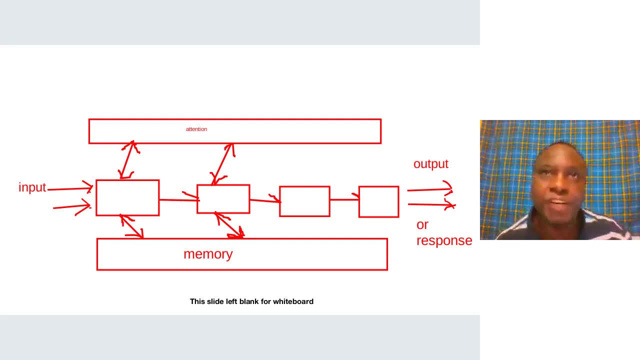 matter of a fraction of a second. uh, you know, from from the input to the output. of course there are some things that may take a little longer, like deciding to run, and you know, but the decision to to run may come very quickly, or at least one. the one which will come past is actually the fear. 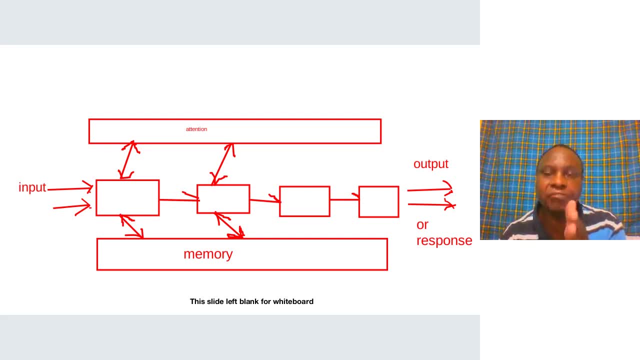 you get fear of, that is going to come very fast, in the split of a second. so this processing is not something that is going to take, that you know, a long, long time. although you know they are doing the diagram, they are saying the first stage, the second stage, third stage, fourth stage and it looks like a long, long uh finger. you know. 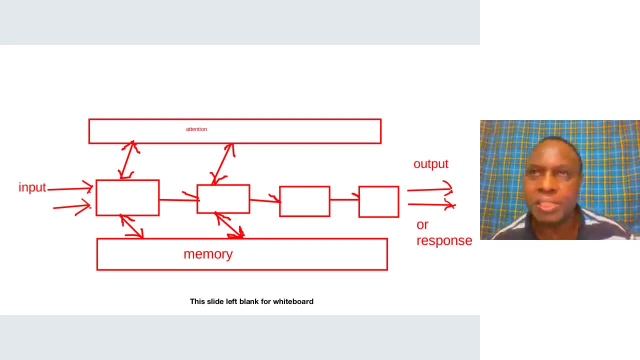 processing stages that it is taking. no, no, it may not take that long. this, in the split of a second, it has already moved from input to output. uh, well, i don't know whether i have been able to bring you closer to understanding, uh, what your question is intended. a quiprop, you could write it again, just in case there is a more. 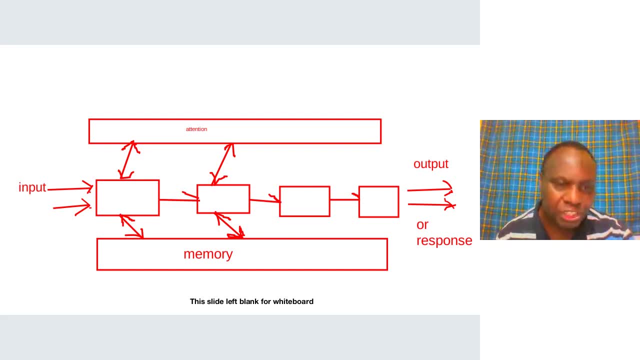 clarification we can put at your question. uh, all right, valerian is also uh, responding to that question. and as for their, since hci could be varying in different service trees, uh, information, maybe guest, guest, a user or service details, etc. uh, all right, and the key prop. 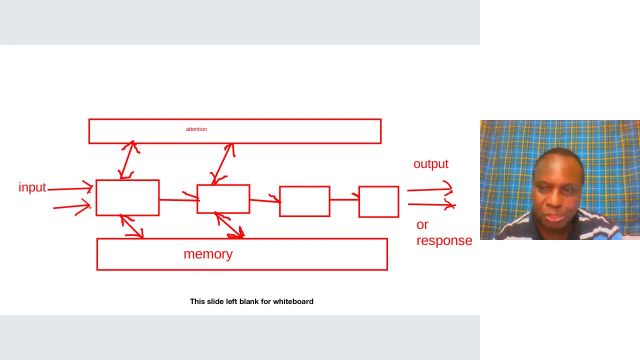 is also responding there. uh, that, uh, you feel clearer uh, what that in is all about. so these are four stages. uh, maybe, uh, something that happens is a split of a second. uh, you can imagine, for an example, if, uh, by mistake, uh, maybe you are talking. sometimes you get animated when we are speaking. 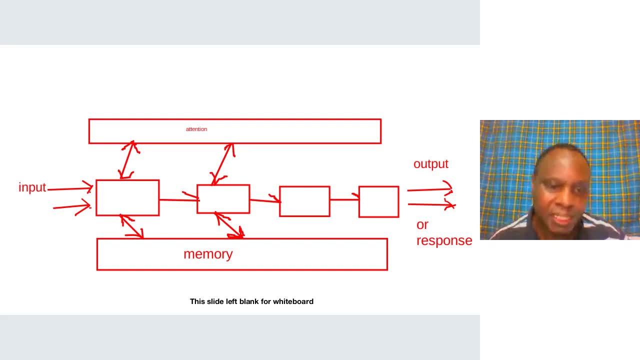 you are in a middle of a a hot, a hot debating and then we, they have to realize that you're near something very, very hot. you just stretch your hand and you, you find your figure on a very hot service. you know, you can imagine how you respond to that. it's in the split of a second. you just say: feel it. 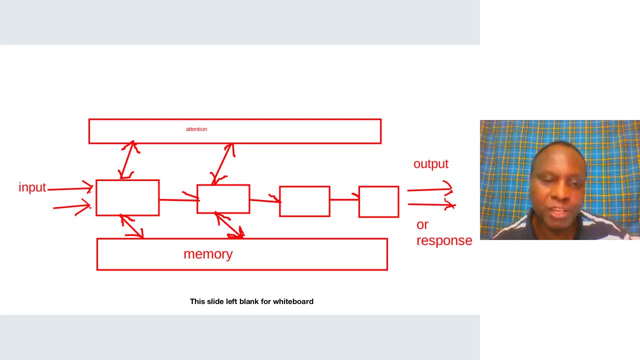 and then you can quickly remove your finger. of course, the first response is that the first output is that you, you, you, you feel the heat, you, you feel the heat. you realize that this is a hot thing, it can destroy me. you know it can burn me so immediately. so, you, you have your finger there. 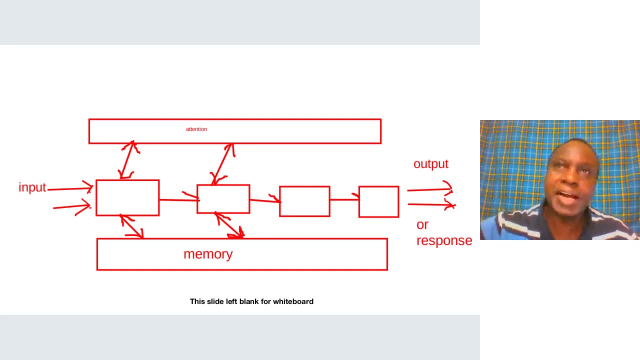 you sense the heat. uh, it's already, you are already, uh, having an output there. uh, so the heat, you feel your finger. so this is a sense of touch. i think that's the sense of touch. you touch and you are your finger. it feels the heat. so this is something that is dangerous and you, you quickly process that. 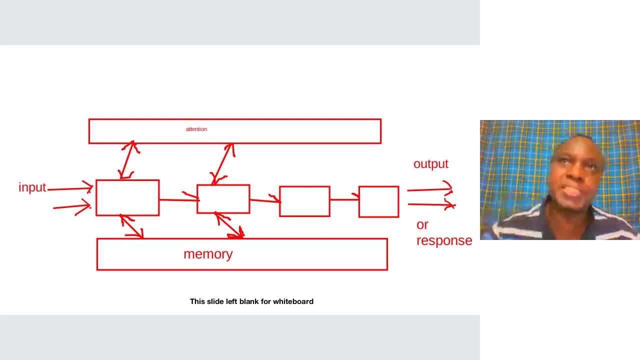 you realize there is a danger here, you pull off the finger. so i think, sometimes a combination of mental reactions and sometimes physical, sometimes it's just mental, sometimes actually you do a physical response. uh, all right, i think then we can go on. uh, so this diagram uh is in the document, the document, sorry, i 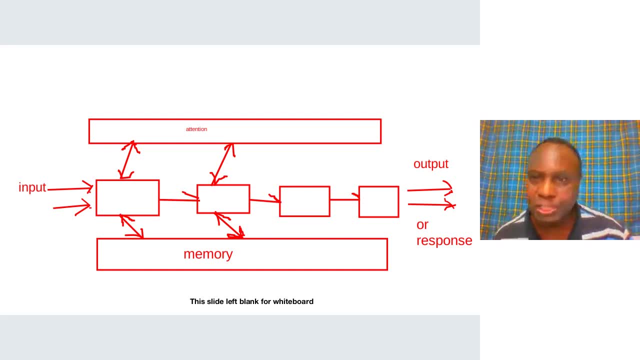 did not put this document earlier, but it is, should be there now. at the portal, you'll be able to see this diagram as part of the document that i have been using for our discussion, and so i, we should be uh today again. uh, i will not keep you for long. i will keep you for a long time. i will keep you for a long time. 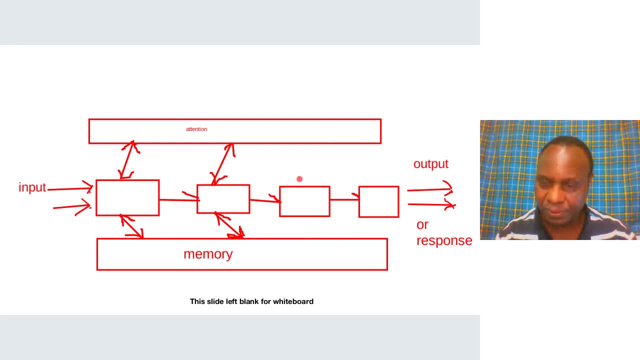 i will like, i will let you, i will allow you some some time of the class to respond to the uh discussion forum for this particular topic. uh so, uh, the lecturer will uh be concluding a little earlier. uh, so let's say, let me share the document again and 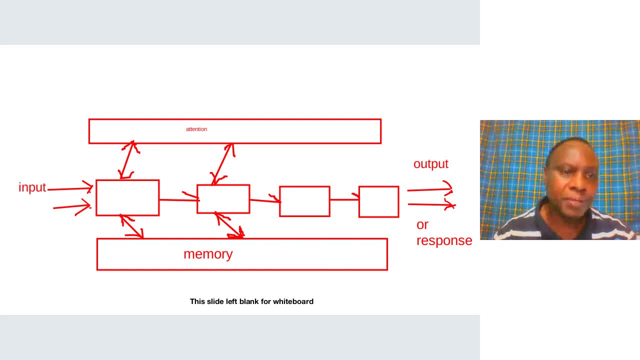 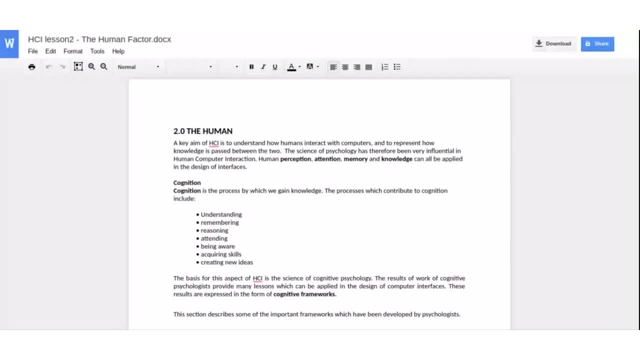 today. we are grateful that the network is working very well and things are quick and also the server is responding very well. so the document is already displaying and so we are looking at at that section where it is talking about the human information processing. so let me just expand it. 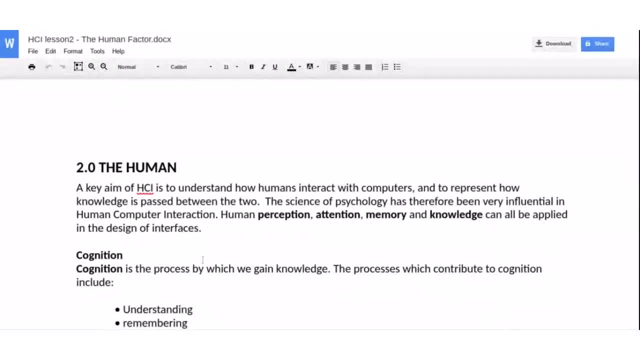 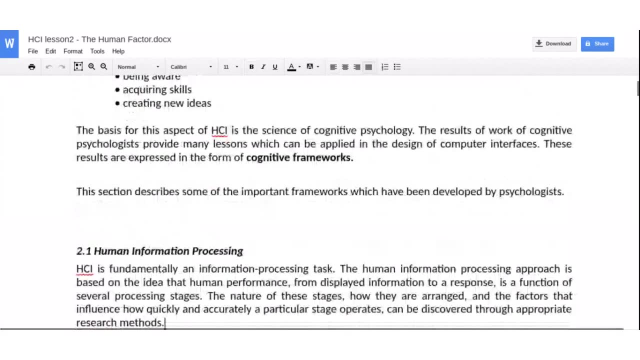 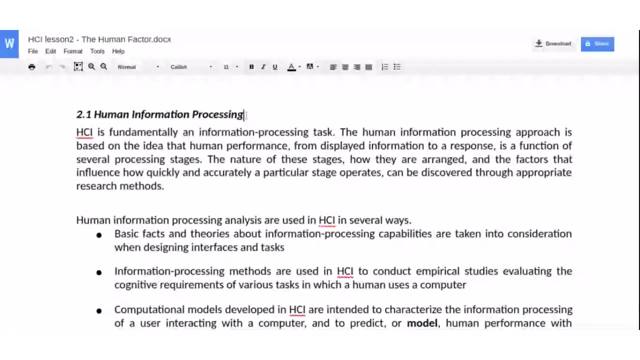 again here and then move down to where we we are. so i had to change to the whiteboard so i can have the diagram. so the diagram should is in the document, but the system is not being able to display the diagram. all right. so we had already covered this portion here and we i wanted to make sure that we are. 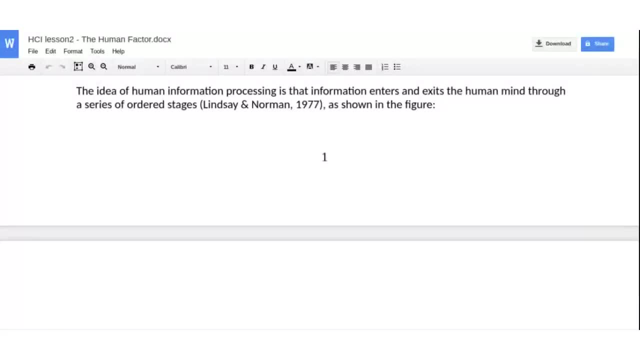 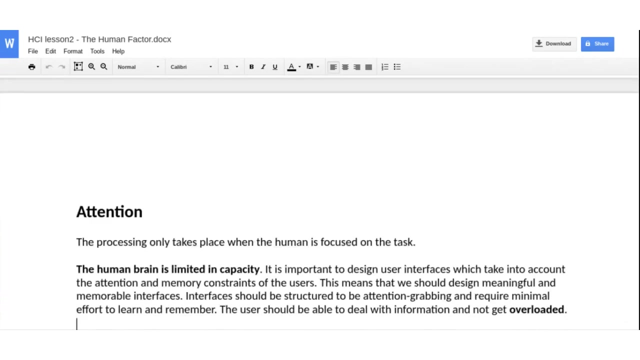 clearer now with the human information processing model and the diagram that captures that, looking at the human as a what we are calling human information processing, uh, or the human is a human as a process, as an information processor, and this we are talking about attention. i think that is also. 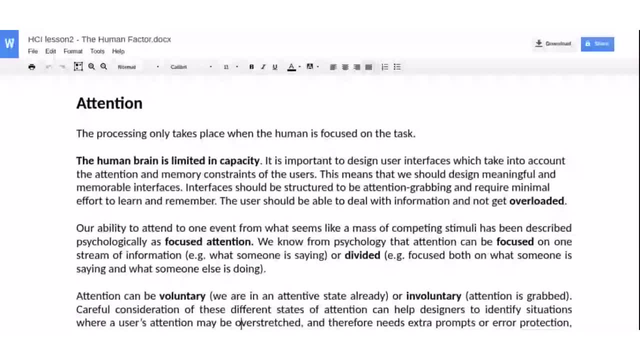 quite well explained. now i think i will let you look at this portion later, but that is a part of what we've uh, apparently i've already explained the importance of attention in the human information processing. uh, you know that whole, uh the stages that uh the information has to, or the input has to, go through. 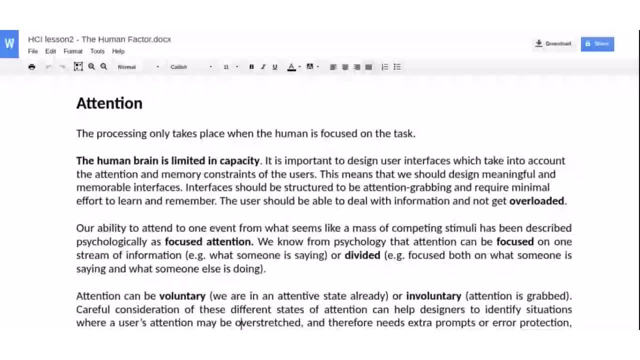 before it turns into what we can call, uh, information as far as the human is concerned, or knowledge in this case. actually, finally, it is supposed to be knowledge and also uh, it may cause us to respond in certain ways. so what is the role of attention? i've said 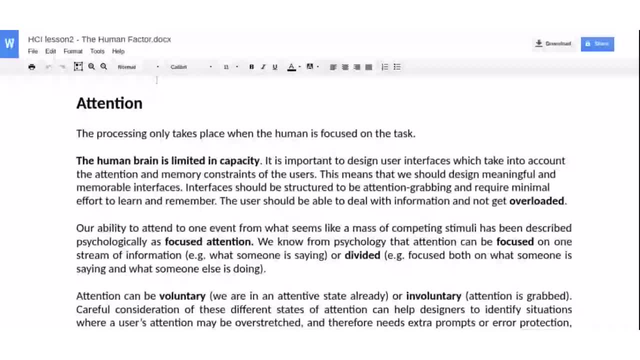 the more you pay attention, then the the better information is stored in memory. actually, this one is, uh is more related to memory. what you can remember is a factor or is a function of how much attention you paid to, to the input. so, for instance, if you are somewhere where some 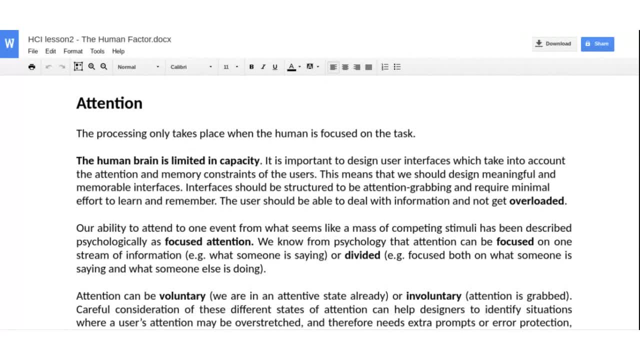 there's a training is going on, somebody is sharing something, so how much attention do you pay? so you're, the more attention you pay, then the better the the information will be stored in your memory, and in that case you should be able to remember better in the coming days. um, so, again, we ought to often. 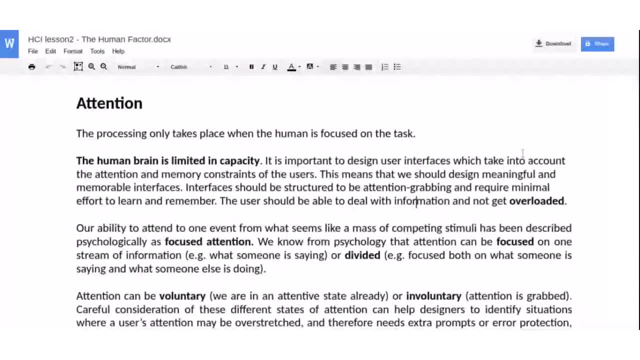 talk about being overloaded, memory getting overloaded, uh, when we're doing certain things again we don't want to now again, uh, now, this is also very important. um, we will need to make sure that, uh, we make it easier to remember things. you know they are. we always need to come up with ways. 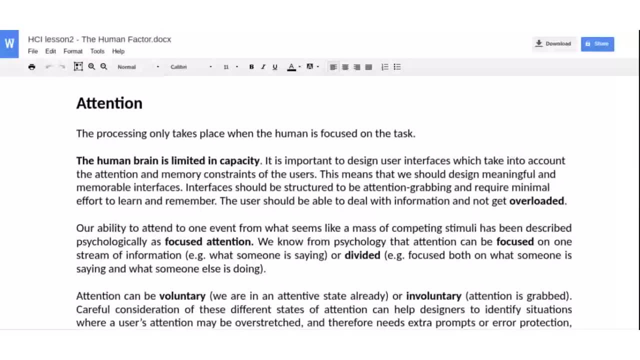 of being able to remember things. of course, there are some things that they nothing that can be done, but, for example, in a teaching uh, it's always a good to keep on looking for uh ways of making it easy for somebody to remember, and that sometimes we always do, but not always, but most of the time. 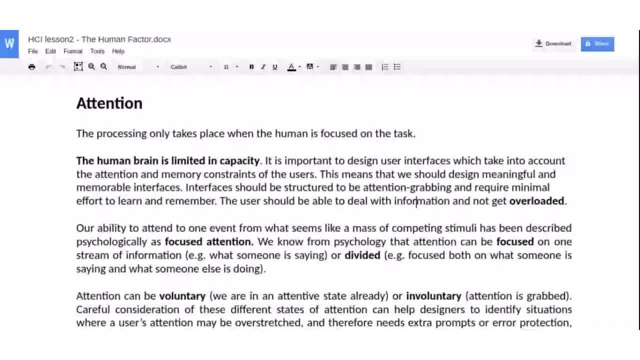 we do, but once, we are not very good at coming up with ways to make people remember something. uh, so, um, but that's a. what we're saying is that, uh, come up with something that makes it easy to recall quickly. all right, um, maybe this one will say later, but is that issue of memory getting overloaded? um, but for now, 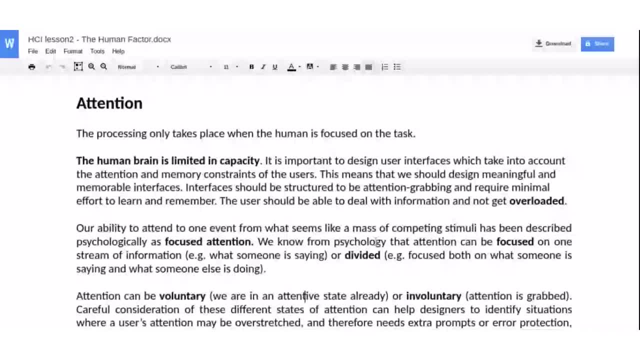 just read that portion later and get everything that is spoken there. again, it's also mentioning about focused attention. uh, so that is where you focus on something that is focused attention. but attention can also be divided sometimes. you, you know, can imagine, uh, sometimes we do that. uh, we try to listen to what is said in different 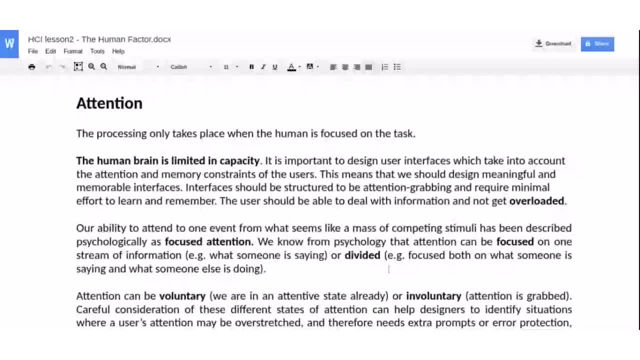 different times. so, for example, if you are now looking at a program in the tv and somebody in the house is trying to to talk to you, you know that is a kind of- uh, divided attention, so you're trying to listen to both. you are still going on. 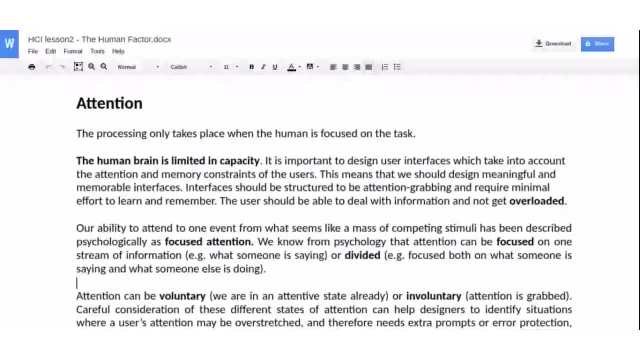 looking at the program, the tv, somebody is trying to speak to you. you know that is divided attention, so you have to kind of uh decide, uh to do focused attention where you decide. now letting me focus to to this. so, of course, if somebody is speaking to you in the 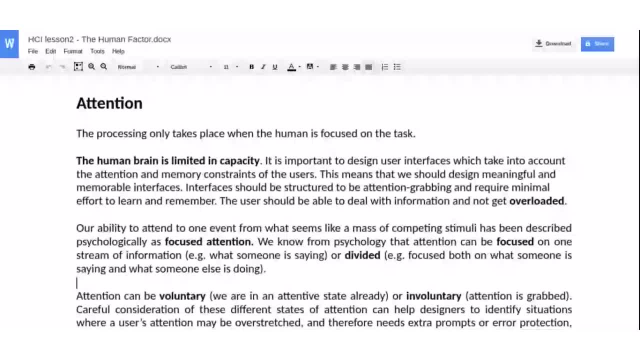 house. uh, of course, the right thing is to first of all, uh, switch off from the tv. uh, pay attention to the person that's speaking to you in the house. uh, you know that now becomes a focused attention. so there is a the concept of focused attention versus divided attention. again, attention can be voluntary or involuntary. uh, i'll let you look at. 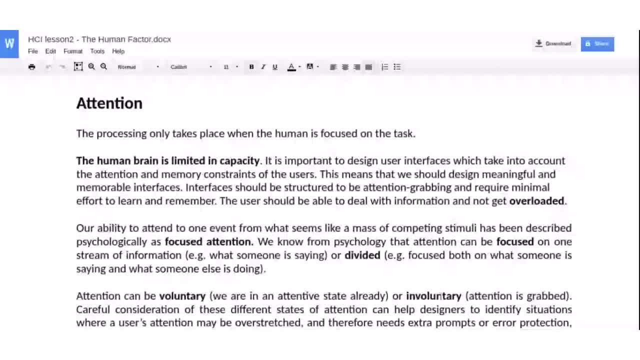 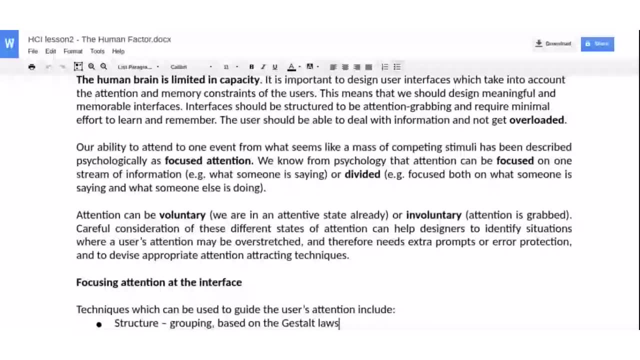 the document and make sure that, uh, you are familiar with all these concepts that seem to be related to, uh, to attention. but, uh, this is also important up here. the human brain is limited in capacity, okay, so we may not always remember everything. in fact, sometimes there's some things that we are trying. 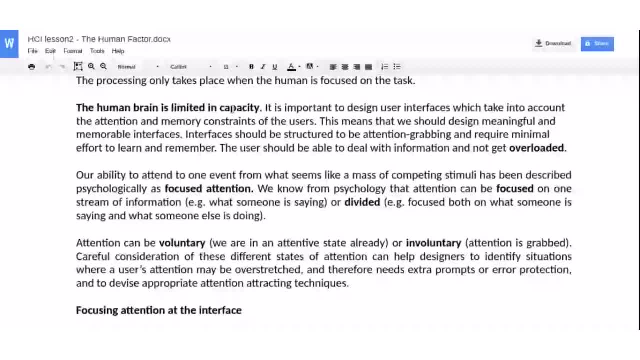 to put in our memory might cause us to forget some other things. now that one is quite difficult for me to explain how that happens. uh, you know, how do we, how come the we say the human brain is limited in capacity? of course that is a fact. but let me 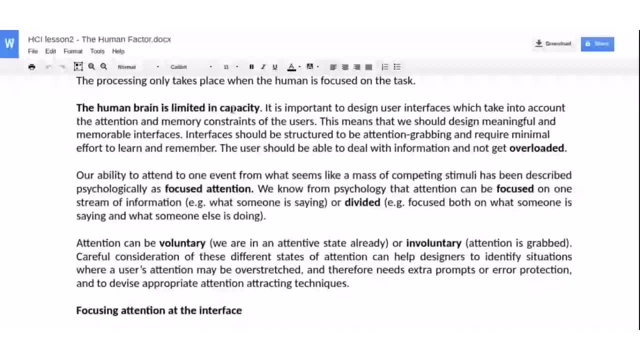 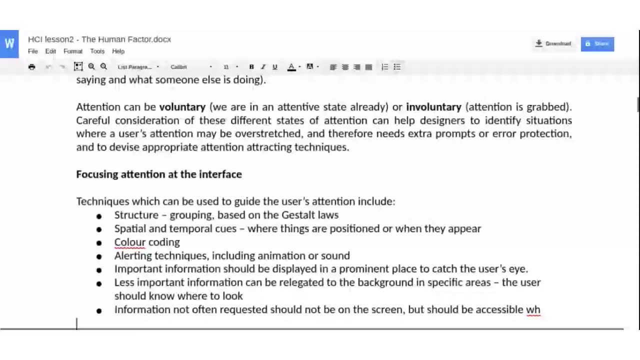 talk a little bit about focusing attention and how that happens. i want to talk about that as well. i have talked about how, uh, i have experienced people trying to focus their attention but not attempt to explain how that happens. okay, so, um, focusing attention, uh, to the interface. 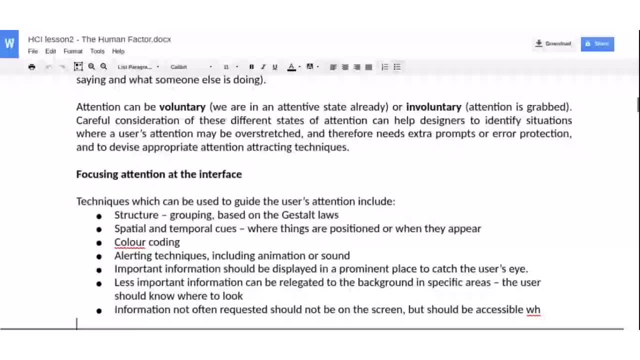 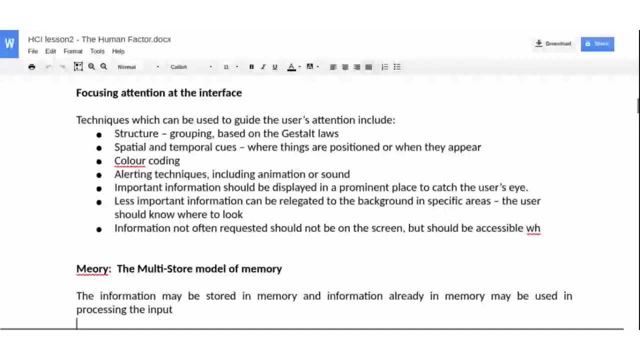 so, um, when it comes now to the interaction between the human and the computer, we have to attracting the human attention, of course, as we're looking at this computer screen, and of course we also learning something from the screen, getting to know where that type of an icon is. when i want to both phase my text, 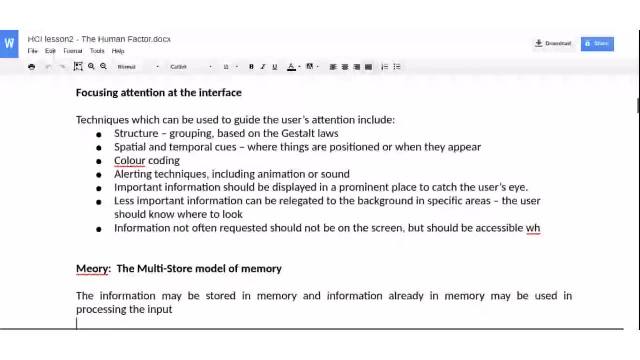 where do i go when i want to save my document? where do i go? you know that has to do with, especially, icons. uh, so how do you, how do you remember all these? and so this portion here is trying to uh, take us to that sees that techniques which can be used to guide the 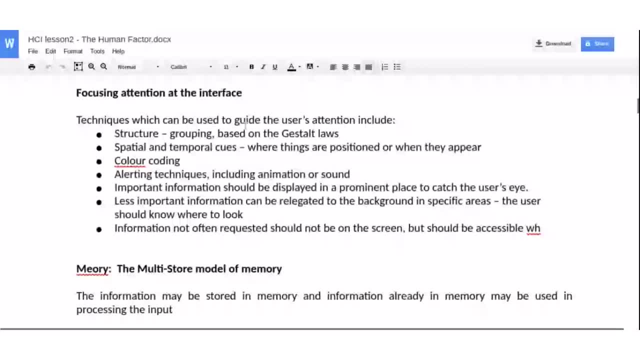 user's attention include what uh include how we structure whatever we want the user to to to notice. so how we structure, that is a concept called the grouping concept, uh, which came up with what is called guestlaws. now we'll be looking at this later in the 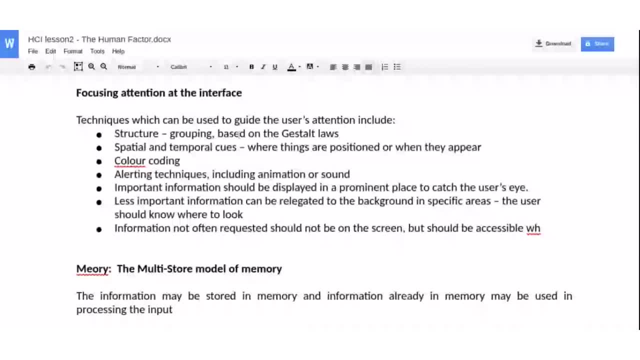 study, um, so you can have a special and the temporal cues that can help in that color coding. alerting techniques: you know, when there is an alert that comes up, uh to help us to pay to, uh kind of uh, uh it wants us to be at, to be at, tend to pay attention to something. 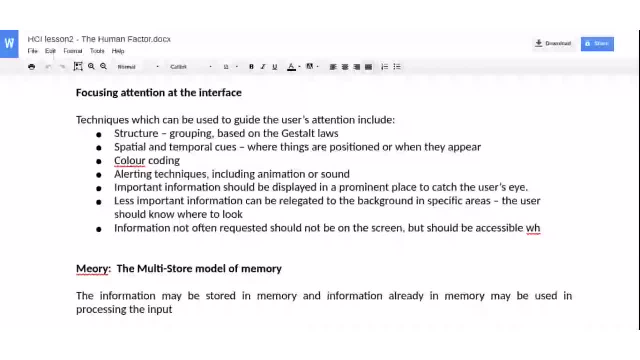 so that there could be an alert, maybe a sound, maybe an animation. so these are some of the ways, some of the techniques that we can use to attract attention of the user at the screen. so we need to consider how do we attract the user's attention at the screen and what are some of the things that we need to do to make it easier. 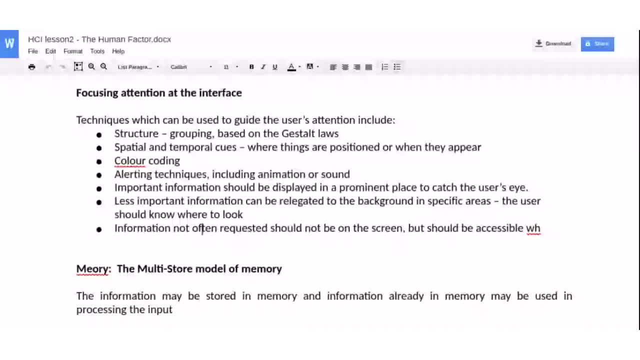 for the computer user to be able to know what they need to do when they come to the computer. we try to do is so that the interface itself, the interface itself, has ways of making the user remember, rather than the user trying to remember from their own memory. we put something at the screen that 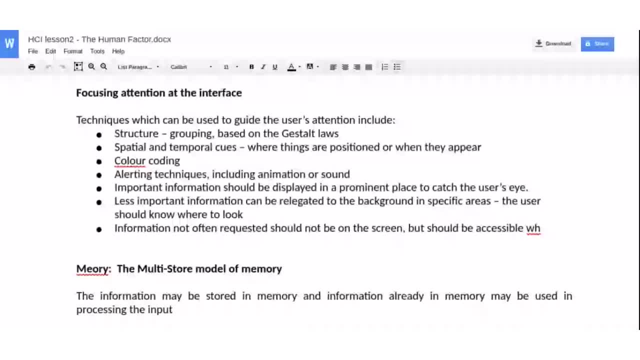 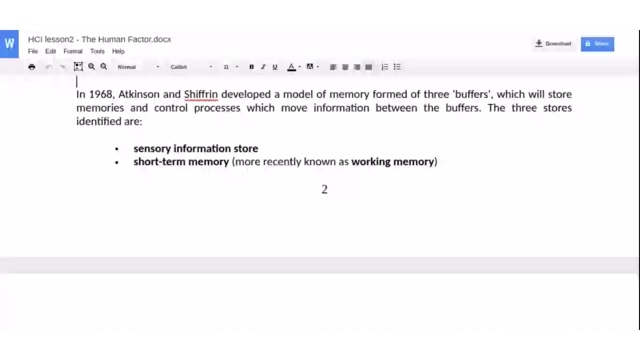 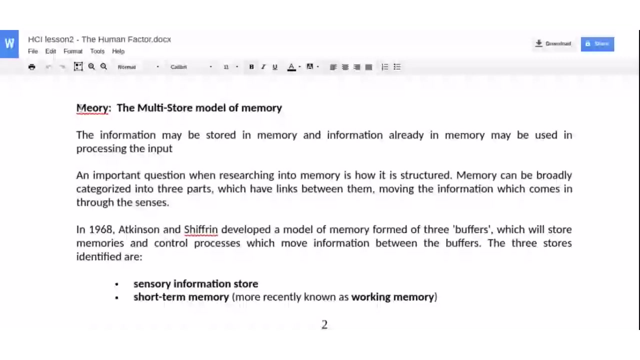 helps the user remember. so you'll be looking at that concept later on. the reducing memory overload: all right, now I delete something. here is a these area, here these are heading, and I think I deleted the whole statement here by mistake. this should be reading the human memory, memory, okay, memory. I'm trying to. 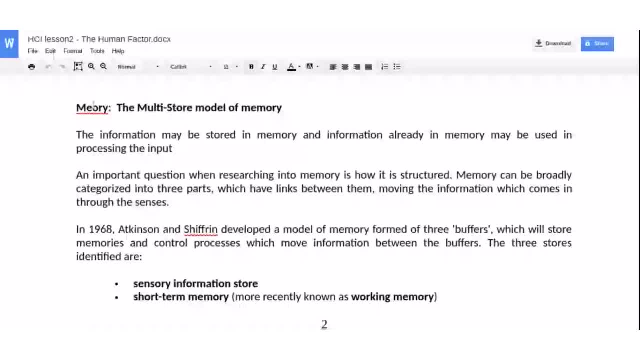 put in there. but okay, now again from the diagram, we talked about the memory and although that's a different model, so the other model is human information processing, but it is another model here which is called the multi-store model of memory, the multi-store model of memory, which says that memory can be looked at. 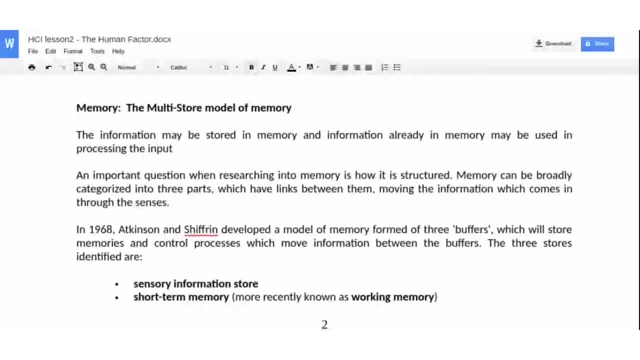 as having three components. three components. of course, these are not physical divisions, but it is. it seems to work. it's like we can look at it as having three components, what we are calling the multi-store model of memory, and the researcher that came up with this one uh. down here it says uh, it is a two uh person who researched on his concept. 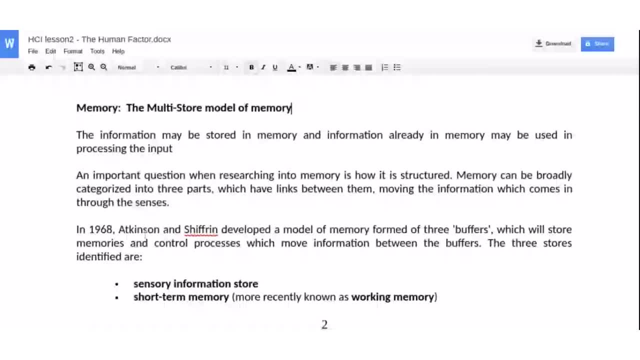 says that in 1968, Atkinson and Shafrin developed a model of memory, of rebuffers, memories and control processes which move information between the buffer. so for them they are saying that, when it comes to memory, we can look at memory as a comprising of three stores. 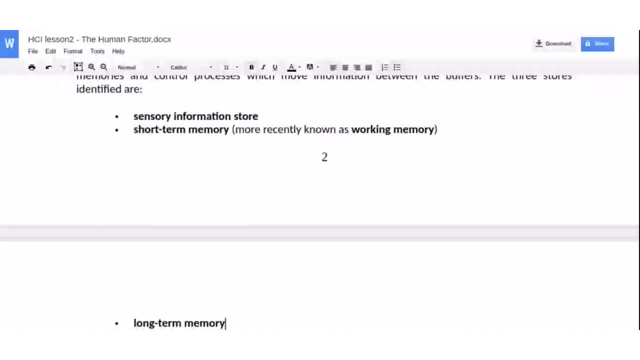 of three, uh, three buffers. now the word buffer- again- I want to believe that, uh, you're familiar with the word buffer above- is like a store, it's like some area that you can store some, some, some data before it can move to another point. it is C? uh, especially during the processing, uh, when it is not storing in hard disk. 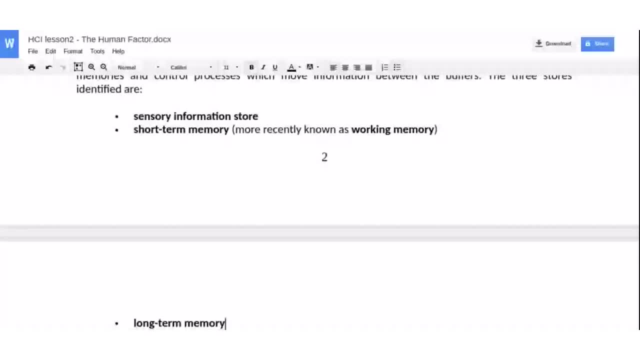 and all that. so when it is just in memory itself, uh, so we have what we call the buffers. so the three uh memory stores are the sensory information store, the short-term memory, which is also called the working memory, and also the long-term memory down here, uh, sorry, my. 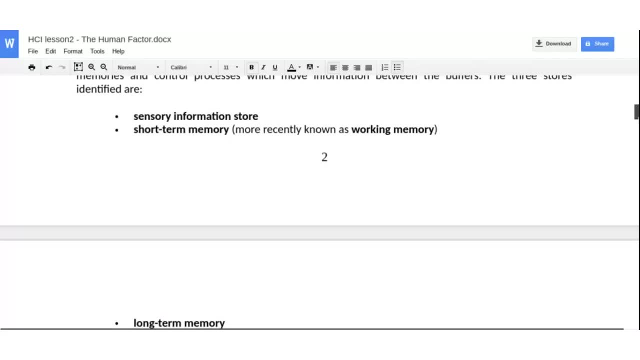 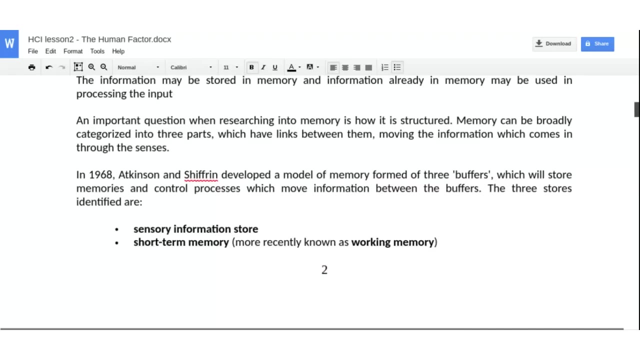 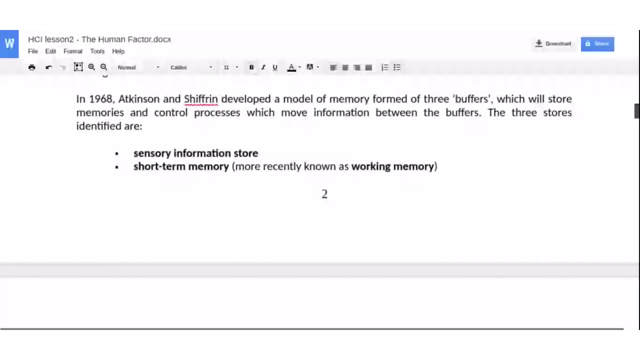 uh. this one is a bit low, so that uh memory store is a long-term memory, so memory can be considered to consists of three uh three stores: the sensory information store or just a sensory store, the short-term memory, uh, or a working memory, uh short-term memory, normally shortened as STM, and 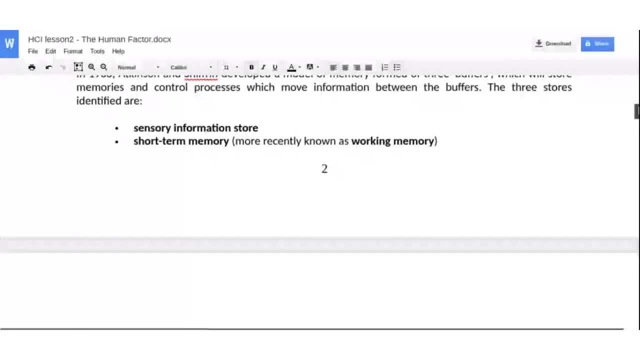 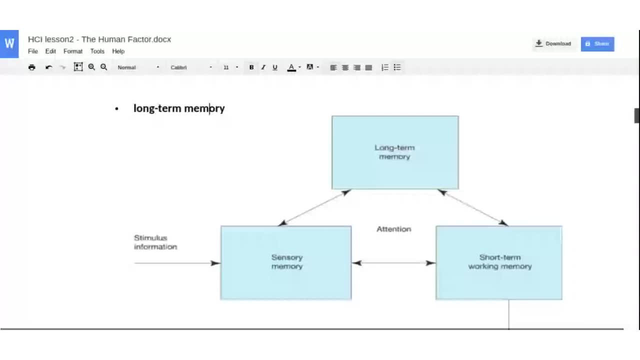 that memory uh store called the long-term memory or the, in a short LTM, and this diagram uh tries to capture that. for some reason this one is showing here Doug the diagram, I don't know why the other one could not show. so this one is showing here, diagram of um, trying to capture that concept of. 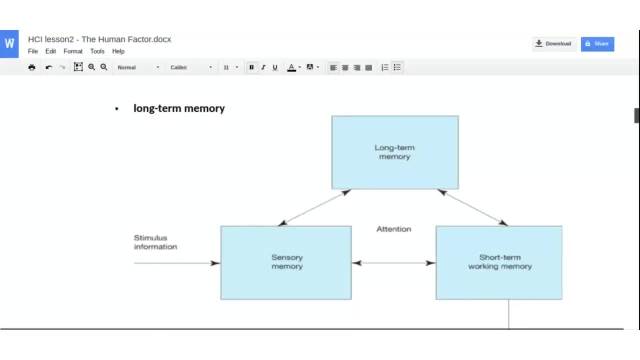 memory as consisting of three different uh uh- memory stores. so that's why it's called the long-term memory, the buffers, the sensory memory, the long-term memory and the short-term memory and says that, uh, so the central memory is where the input is interacting with the sensor, the senses, so like. 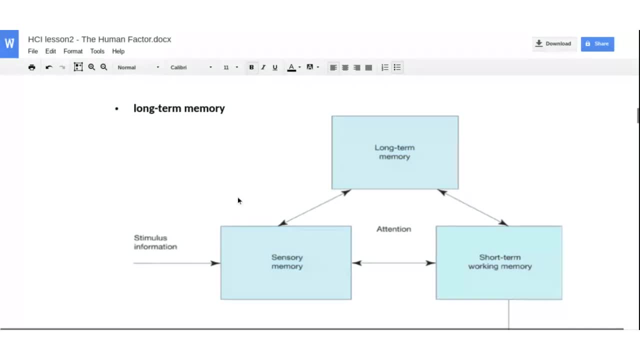 well, we were saying, for example, touching a hot, uh, a hot object, so at the point where you you, you turn, that's the sense, uh, so the information, uh is the input is coming through the senses, so the stimulus is coming through the set, so that, uh, what experience at. 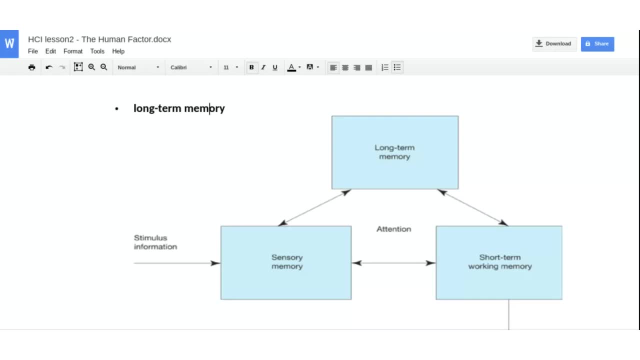 that point is being stored very briefly. are there the sensory memory? but if you pay attention it can then go to the short memory. so the short-term memory is when you are now, uh, paying attention. then, uh, the uh, whatever you are paying attention to may now get. 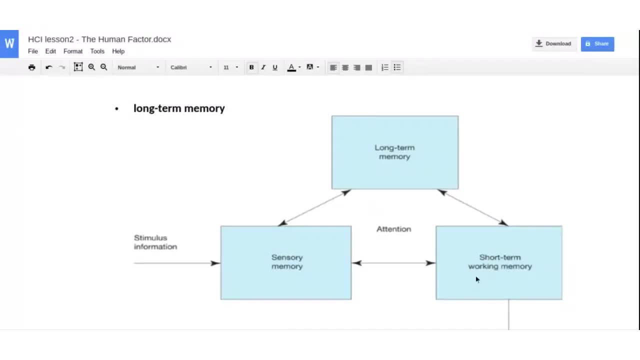 stored in the working memory. so that's a like when you are meditating or when you are paying that attention, then you are allowing- uh, you are, you know the process- to proceed to the short term, uh, what we are calling the short-term memory or the working memory, and 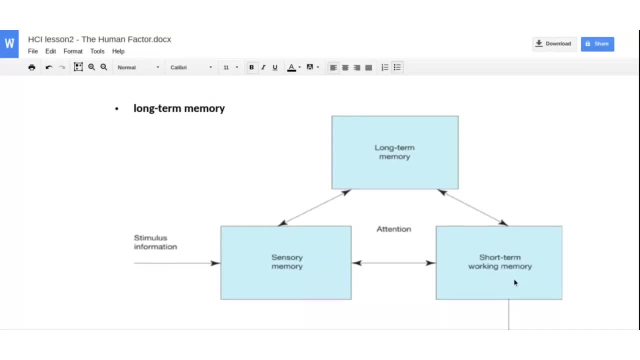 it is that if you continue to bring that attention for long enough, then some of what has come to the working memory can actually proceed on to the next level of memory, the long-term memory. and this authority says that, uh, when something goes to the long-term memory, it is almost permanent. 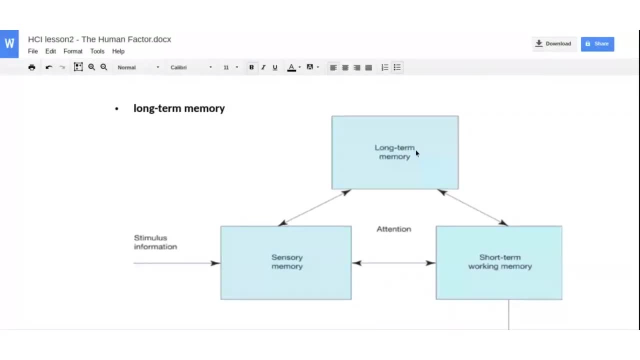 you can remember it for a long, a long time, and I'm sure each of each one of us is likely to be to recall something that we can remember but which we actually with them. The first time that we are interacting with them is a long, long time ago, Or, of course, 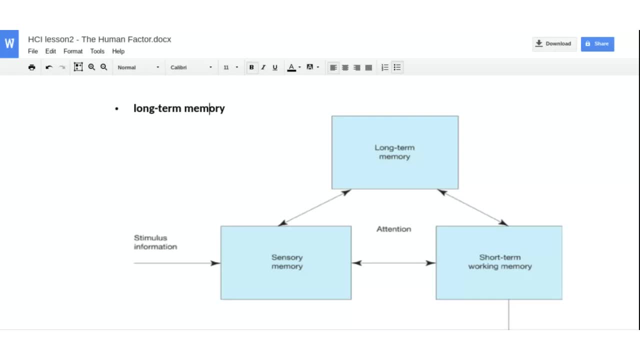 maybe it's something that we have been doing now and then and therefore it is becoming part of, maybe we can say part of us, Even if I later now stay for a long time without either hearing or seeing or being physically doing that particular action, Maybe like the trained, as we said, you. 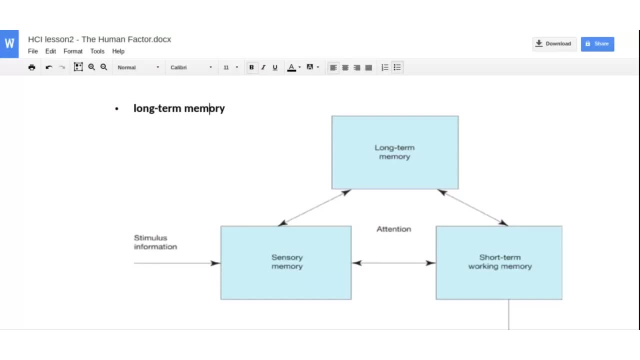 find that you can still recall, and I'm sure even with the training, I think, some things like in sports. I find that somebody may not have been doing their game. maybe they are. they are they are footballers, They are, they like football, Maybe they have been playing football or even if they probably take some span of time without playing football anymore. you know, for a long time when they say no, no, i have decided to go back to to playing football, you find that actually they can. they are likely to pick up and become a just as good or probably even better than than previously, because it is something that 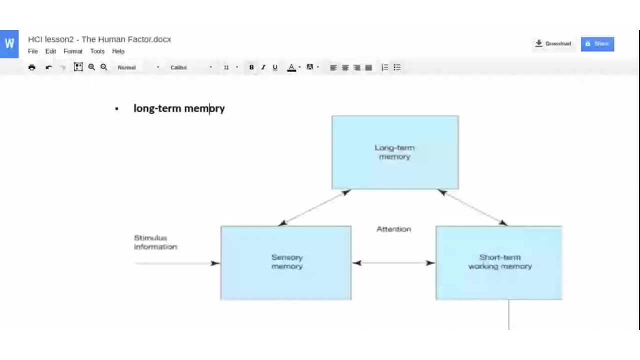 they have done. it's a kind of type a part of them. but especially in terms of memory remembering, uh, you find that, uh, if you have not, uh there's a place that you have lived before and then you, uh, you move to another place and then, yeah, for a long, long time you've not gone. 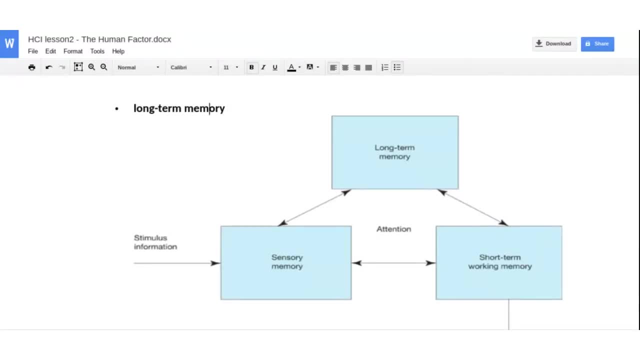 that place before. and then you decide, oh, let me go back to uh to maybe see something in this place where i used to be. you find that you can actually so easily remember your way around, of course, and this could have changed, and yet you can remember the exact place that. 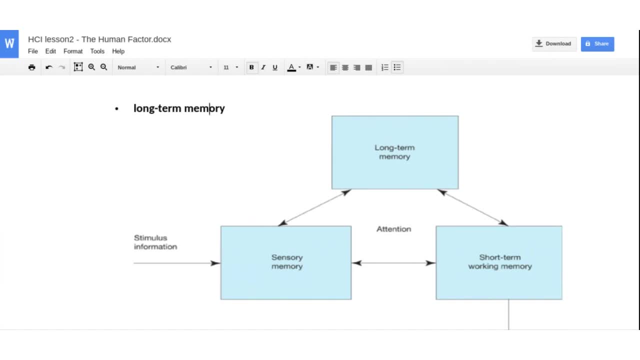 you want to go and which you have not gone for quite a while. it could even be several years, and yet you are able to find your your way around because you are remembering. so he's saying that, if you allow, uh, when something has come to the uh shorter memory, uh, it is uh. 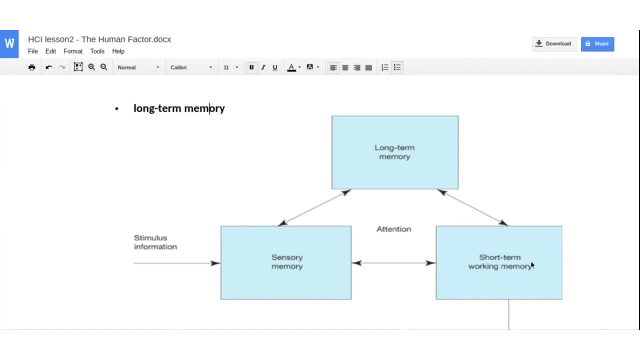 very, very likely that you will end up into the long term memory and then it means that you can. so you know the viewers have said uh says that if something comes to the long memory then it is almost permanent. it can be remembered for a long, long time in the future. 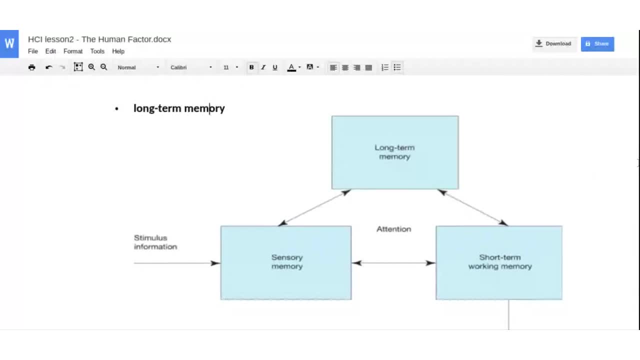 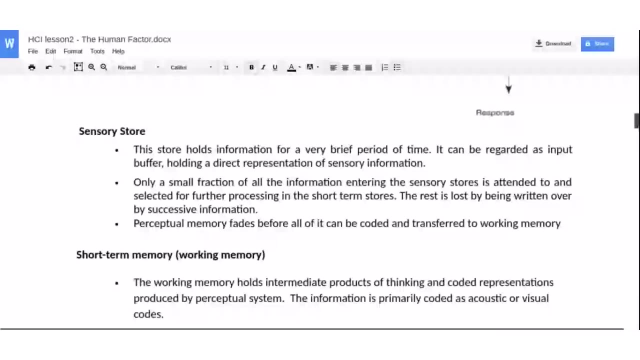 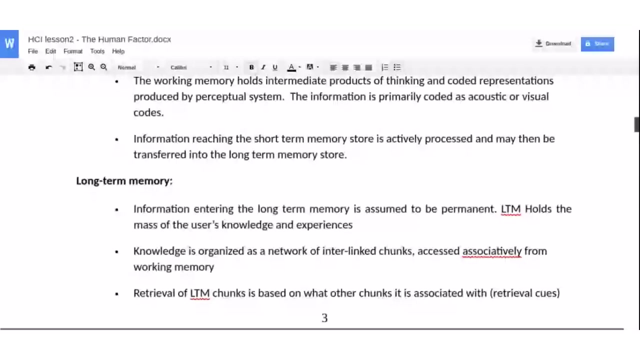 um, so i think for today that it would be sufficient. so please read the text. i have not uh gone through the text with uh, with the class uh. please look at the text so that you can capture anything that i have not uh brought out in the in trying to explain the the three uh memory store. 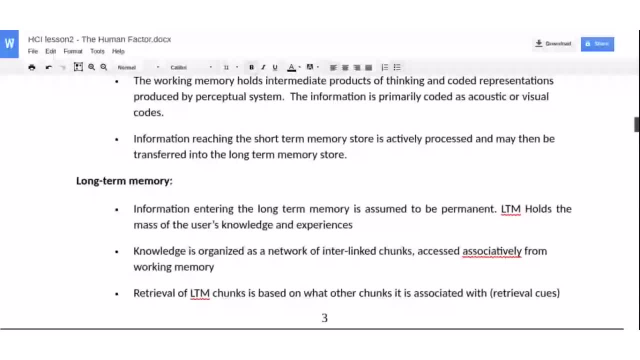 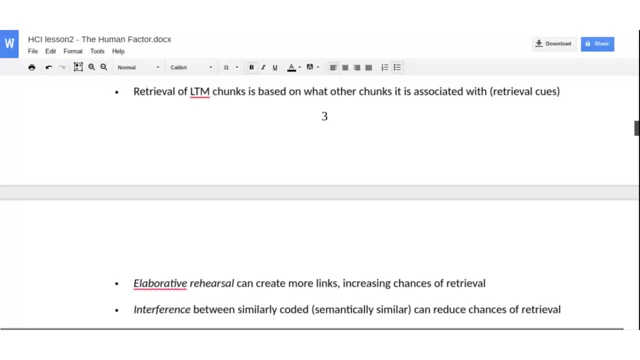 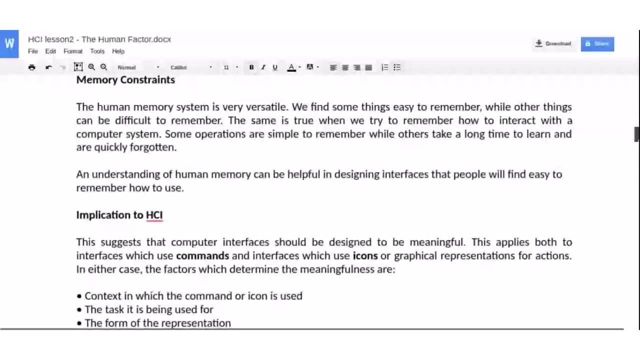 model or the restore model of memory. the restore model of memory? uh, look at the text here and the issue that uh is very clear to you, how you can explain uh, the restore model of memory. so, as we had already mentioned earlier, is that memories? you know there are challenges. memories sometimes it's not. we can't, of course, remember. 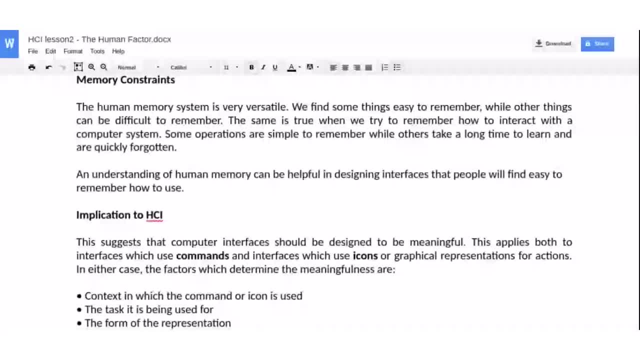 everything. sometimes we forget, and so what are the implications of that? uh, so it is stated here that we need to do a few things to help a human to interact with the computer, because some of the the user has to do has to do with the remembering. so, for example, if you are trying to, as i had, 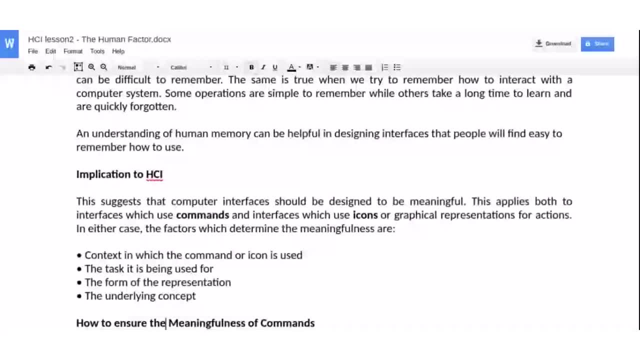 said earlier, if you are typing a document, it's a place where you want to bold face your text. now, that calls for remembering. so where is the icon? what uh, what command? of course, in this case, we are dealing with the uh using these graphical user interfaces, so it's likely to be an icon. 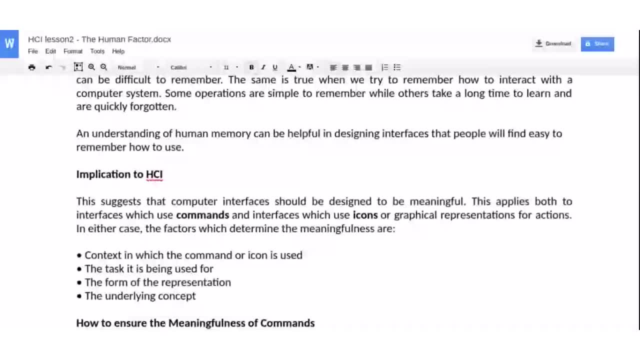 so how can you remember the icon what? what can help you to remember anything? so the implication is that we need to come up with some ways of helping a user to quickly remember the functions that they need to use in order to be able to accomplish their tasks- the tasks they 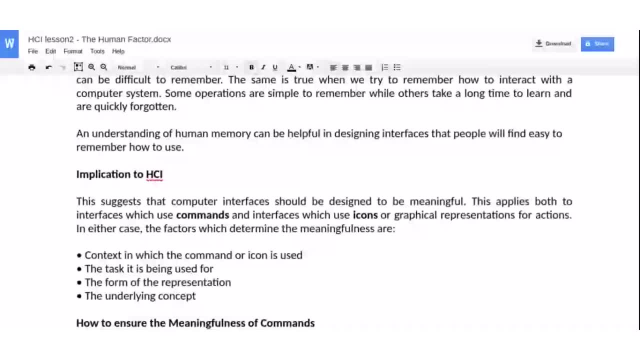 want to accomplish at the computer. and so it says that: uh, this implication. let me read this text here: that this suggests that the computer interfaces should be designed to be meaningful to the user. the computer interfaces should be decided to be meaningful. this applies both to interfaces which use commands and interfaces which use icons, which we call graphical. 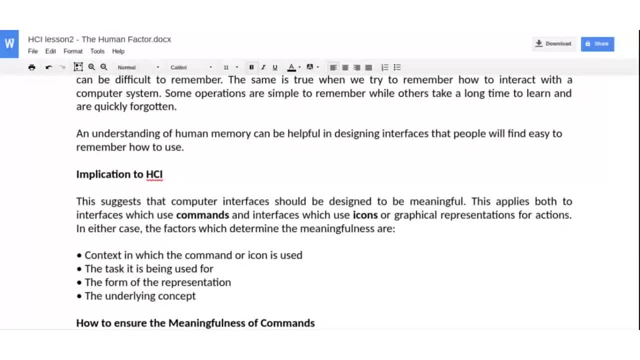 user interfaces and so um, in that context i will read a little bit more of that. but how do we ensure to make commands meaningful? how do we make the commands be meaningful? how to ensure the meaningful, the meaningfulness of commands? so how do we make the meaning of the user? 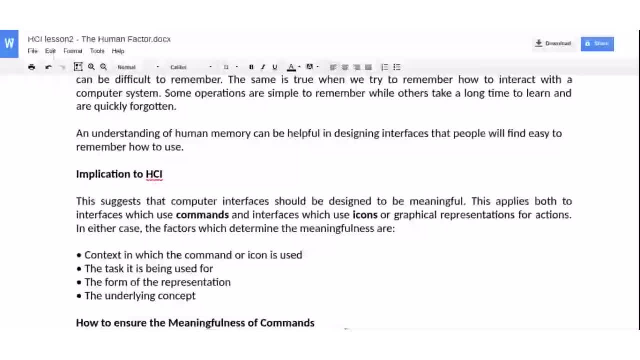 they will make commands meaningful to the user. so of course, in this case we kind of saying: how can we make it easy? if it's a matter of commands that a user has to write, how do we make it easy for the user to recall those commands and be able to use them so that 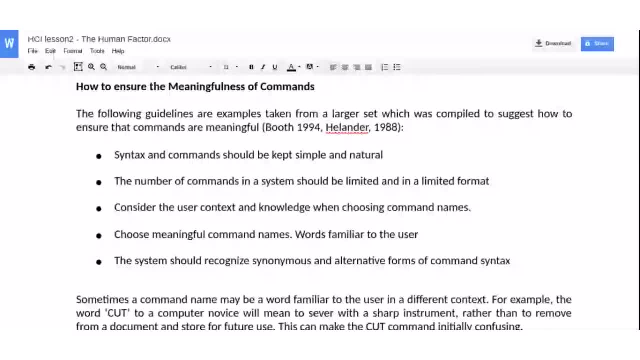 they can go on with their work at the computer and accomplish the goal for which they have come to the computer: to do some tasks, and that is what is explained somewhere here. some of the ways are suggested of making what we are saying to ensure the meaningfulness of commands, and they are. 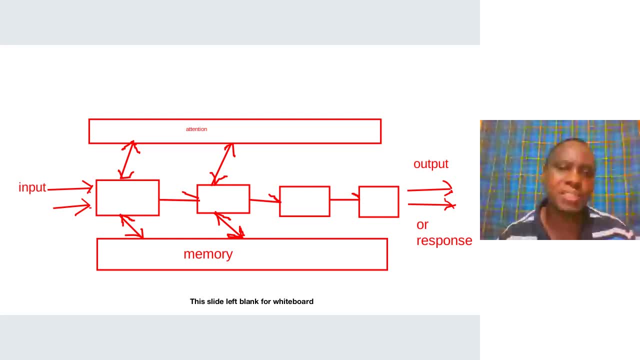 suggested here, for example, the first bullet saying syntax and commands should be kept simple and natural. so make the commands simple. of course, nowadays we are dealing- we are now you more dealing- with the user, graphical user interfaces, but we still once in a while do some commands and once in a while we still have to. 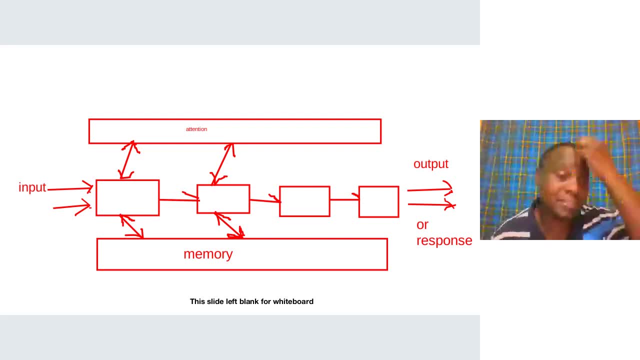 write some commands. so how can we make them? how can we make it easy for a user to remember the commands? and so one of the suggested ways: the syntax and commands should be kept simple and natural. at least a word simple there, I may be easy to recall. I already at least understand. 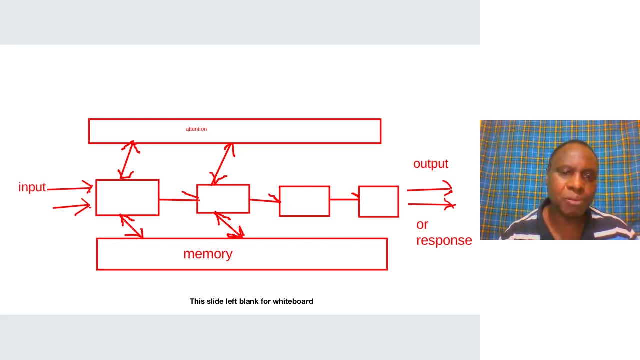 the number of commands in a system should be limited and in a limited format. so if they are too many there some of the commands a user will forget. we try to keep the commands to a minimum unless user knows enough commands to understand. so we try to keep the commands a minimum but sometimes it's. 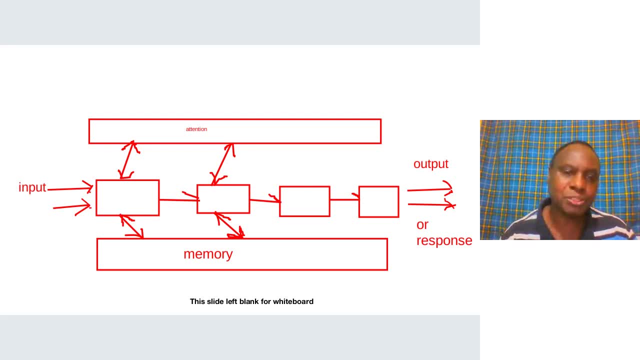 challenge because it all depends again on what the system is meant to do. So please read again this area here and get to fully understand what is meaningful and be able to give a number of suggested ways of doing that. How can you make commands meaningful? 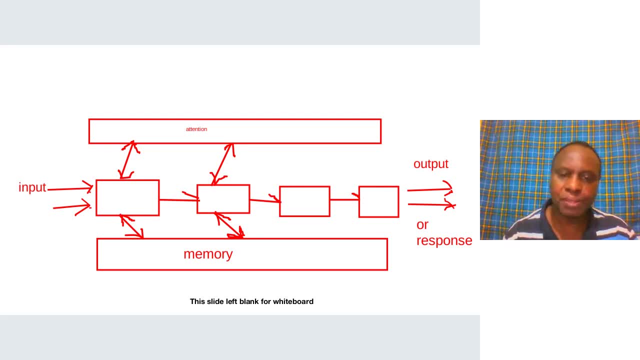 Maybe this might be an important section here. Let's see what it says here. It says that sometimes a command name may be a word familiar to the user, but in a different context. So again we want to make a. So the word may be familiar, but sometimes we may find that in the computer. 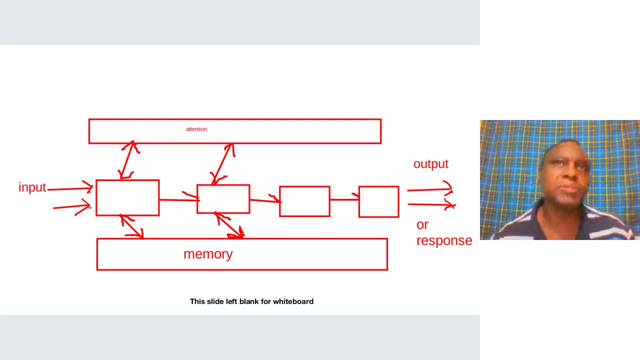 it is used in a very different context To what we ourselves, especially culturally, we are used to, And so, for example, the word cut which we use in the cut and paste and copy and paste, So this word to the computer novice may mean to severe, So I think the word is supposed to be severe. 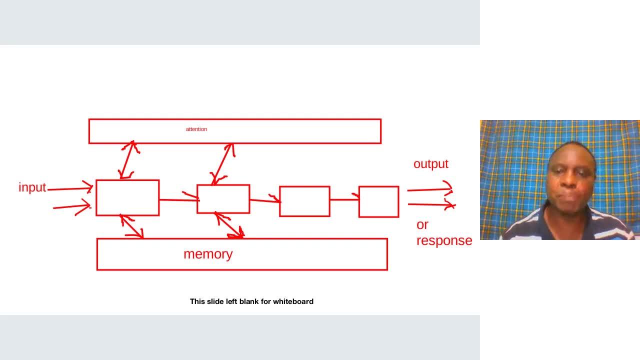 with a sharp instrument rather than to remove from a document. So again, so unfortunately, some of these technologies and the words that they use may be coming from a different cultural context, and sometimes they may not always be as appealing to some users as to others. Those that come from the context. 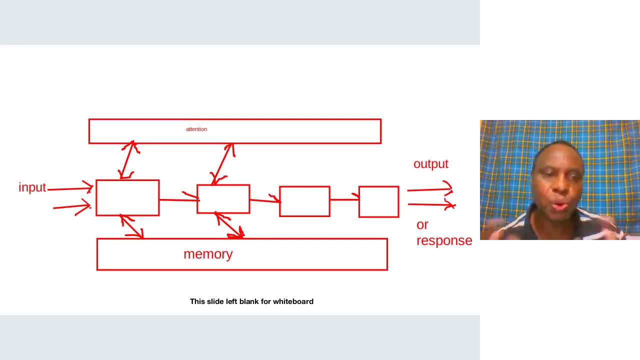 where these word is. they used there in that way culturally may make sense, But to some other people that may not Using the word cut, it may make sense. acutually may make sense, but to some other people that use the word cut some of those words are used in that context. For course also we see that different cultures that use it Of course they may not have different també to available people and some people may like and understand the expression or think or listen to the words. Those are common words and ny kotta even its effect, etc. No, Ciao, guys. 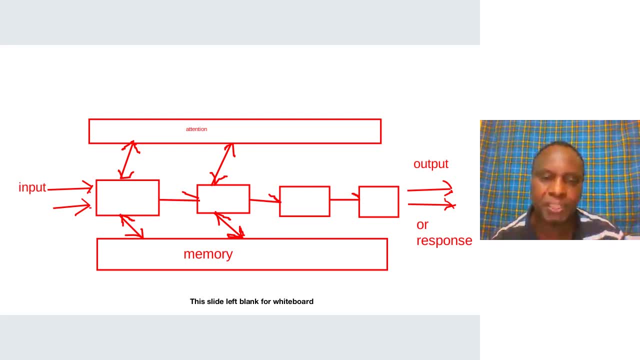 are coming from a different context, it may not always make sense, and so sometimes, of course, we have a challenge, uh, because we are using systems that are coming from a different, uh, cultural context. but again, i think, since the world has become a global village, uh, sometimes we find that 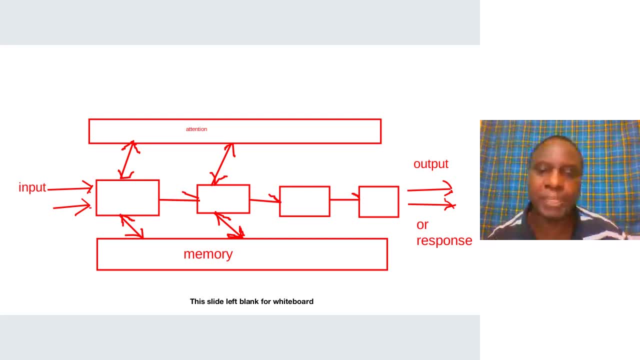 this is helping, uh, that, even if it is used in an american context, sometimes we may have already known how the americans look at this word and sometimes we may figure out, uh, what it is all about, and they not get too confused how to utilize it at the computer. but anyway, that's also an 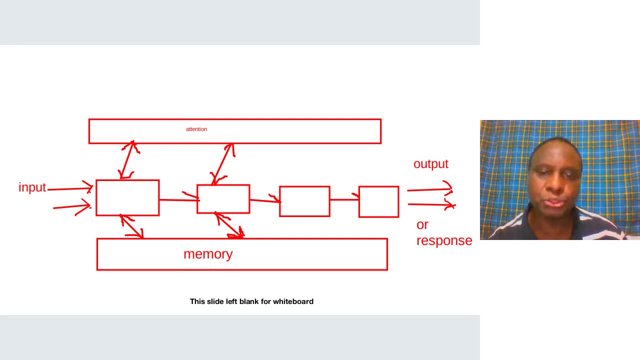 important issue to highlight that sometimes the- the name that has been used in computers, uh- for certain cultural contexts, may actually be confusing to other cultural contexts. i will be coming to that, uh, sometime later and look at what is called the metaphors. we'll be looking at that, all right. what about the meaningfulness of icons? 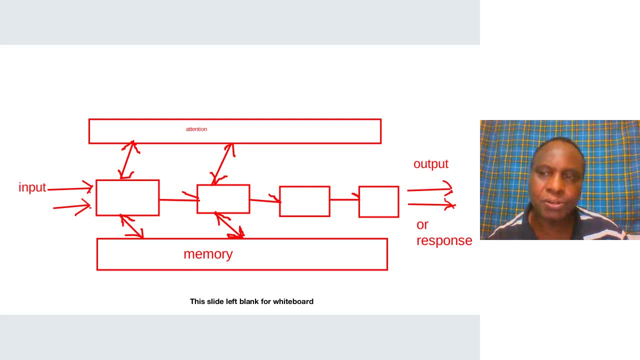 so the icons again also. we also need to make icons meaningful and again here we have some suggested ways uh of making icons meaningful. says here that icons can be used for a wide range of interpieces, for example labeling uh, warning, identifying, manipulating, being a container. for example, there was with with the basket, uh kind of uh, an icon, uh, you know. so there's, as we 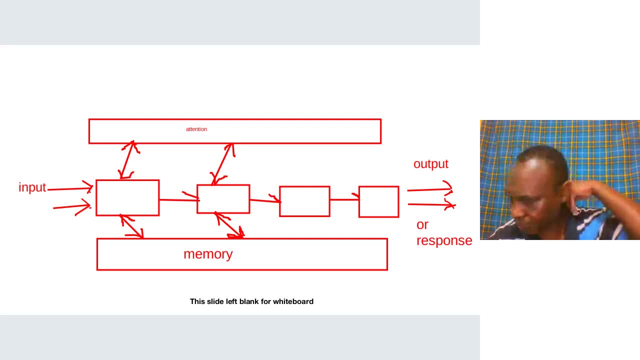 said, as i say there, some of these are based on something we call uh metaphor, and we'll also come to look at the metal, but in the meantime, please, uh what people are daily more interested in. thank you, review that, uh. how to make a. now, these are just ways that icons are used at the computer, but how? 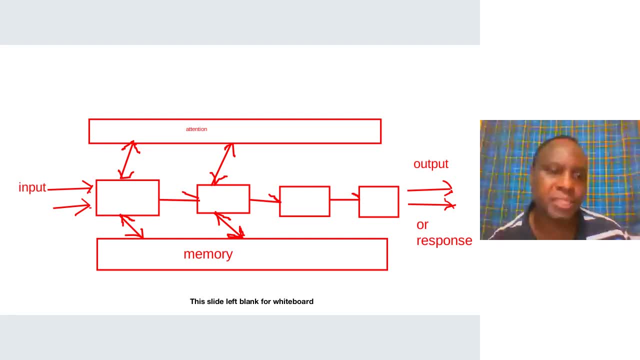 to make them to be meaningful to the user. so there's some suggested ways that down here. uh, i'll ask you to read on that. uh, please read on how to make some of the ways suggested of making um icons to be meaningful to the user. so, keep them simple, keep making them use. a, of course it's. 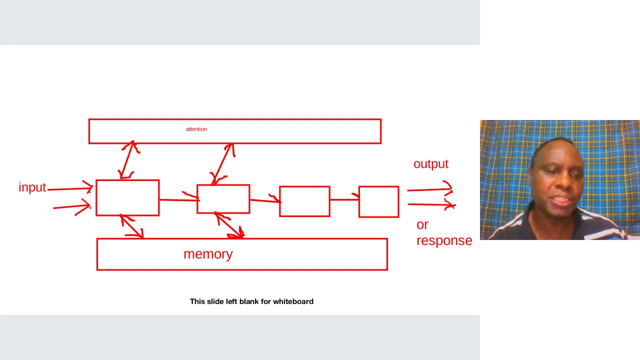 more about. yes, the icon itself needs to also be familiar, but most likely it is the way you label it: uh, of course, the kind of uh, a figure you use for uh, for the. you know the, the, the diagram symbol that you use for the icon. that may also be. 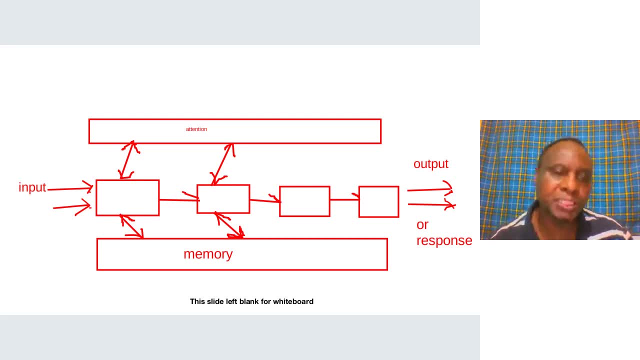 important. if you can get an image that is familiar to the user and it almost looks like like what you are trying to use the icon for, that would be good, simple, familiar, be consistent. so that again is important. but, as i said, look at the whole list, look at this and get to know. 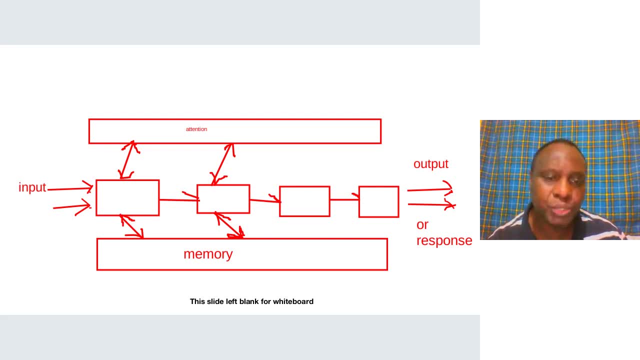 the various ways that, um, you can make icons to be meaningful to the user. um, i want to believe that we have had enough for today, so there is a section here which i want you to also to read on your own. uh, please look at these multitasking interruptions. this is still. 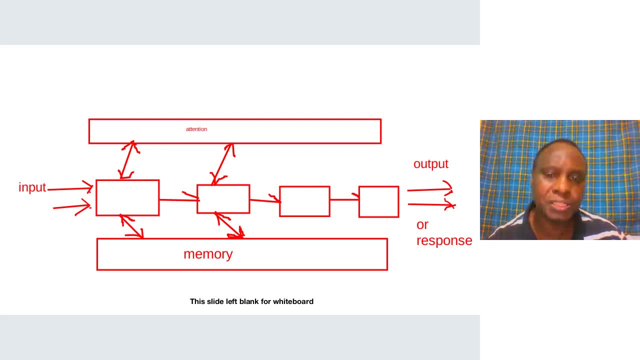 has still to do with the issue of memory, uh, so look at that. uh. issues about uh. how do you handle multitasking interruptions? uh, or what can the the design, the designer of human computer interaction do to deal with the issue of uh, multitasking and interruptions that the user sometimes can find themselves in as they use? 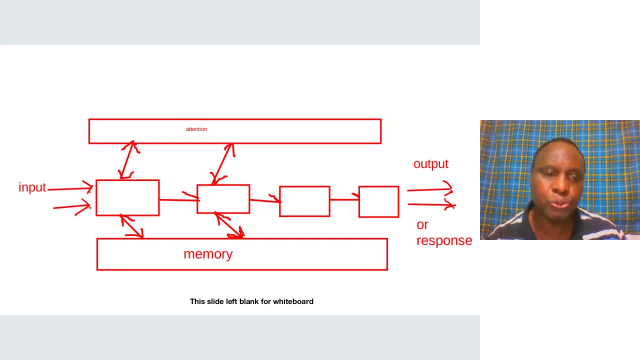 their computer and with that i think we'll reach there for today and the next session will continue with this um, the human uh in the human computer interaction uh study uh. but we go to this section uh talking about perception and issues related to perception as far as the theories in human computer interaction. 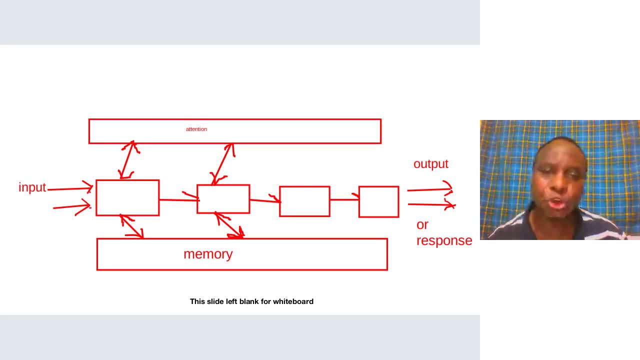 is concerned. so for now, i think we learned, therefore, a presentation by the lecturer, but i want again to just say: allow a moment of interaction. uh, please, you can raise an initial of clarification or a question or any type of comment. so i want to switch back to remove the 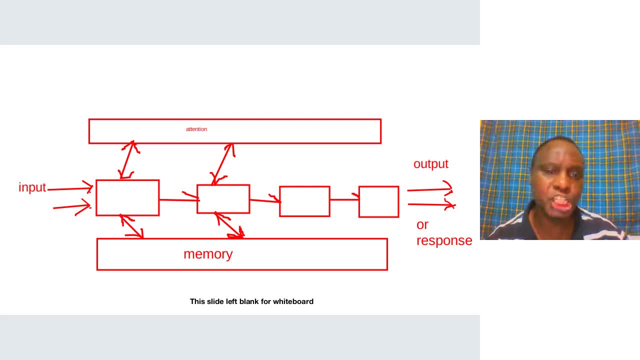 screen share. this document is already at the portal so you can access it there. but i say, as i said, i'll also i'll need a maybe to send a the whole bunch of the notes that i have for this unit to the email of the class rep and 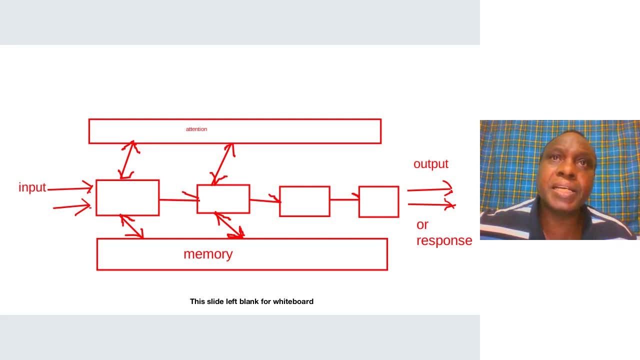 he can distribute to the rest of the of the class in one way or the other. so you can access the. you can have all the notes ahead, uh, but of course you'll always have them at the portal. but they may not be very fast in the being able to put all the the notes in all the topics, uh, because it takes quite. 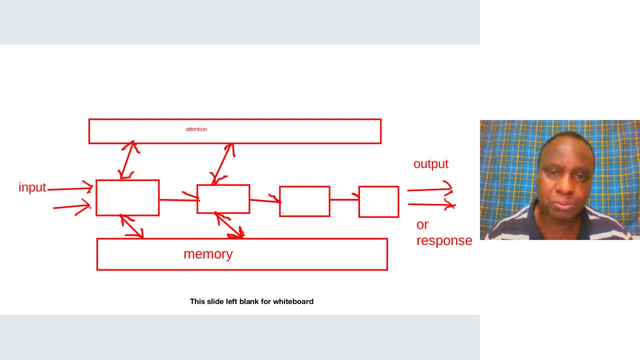 a process to to load at the at the portal, but of course i'll make careful to have this. these notes appear way ahead of the day of the class, so otherwise, uh, yes, so let me remove the share. uh, let me get back to the screen where you can see the image of the lecturer. uh, and i'm waiting for. 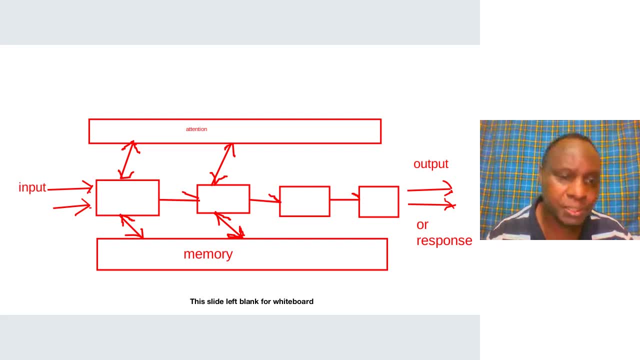 you now to raise any point of clarification? uh, point of clarification. uh, all right, uh, sorry, i think i had already removed them. um, yes, so, yes, so uh, any point of clarification or a comment? uh, please, you can uh write at the chat. i think that would be very uh. 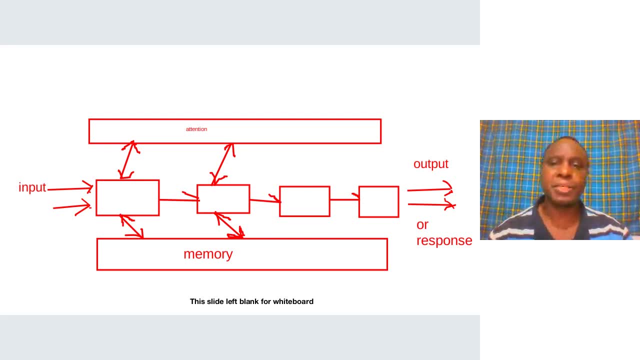 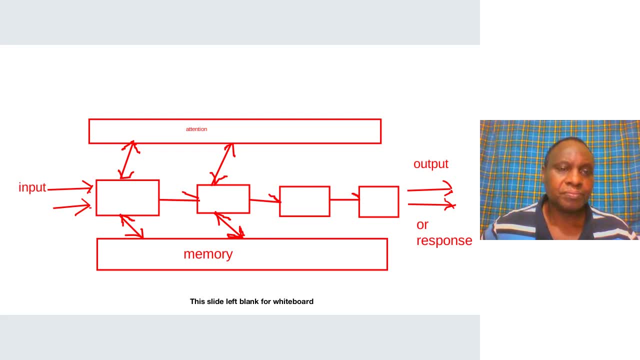 um, um, um, um, um, um um you, valerian, for responding to our previous question. thank you for uh putting your response there to contribute to the discussion. uh, yes, the key prop using the screenshot is not displaying. yes, i have removed the screen share. oh, i didn't. i did not share the screen. oh, sorry, sorry, uh, i forgot. 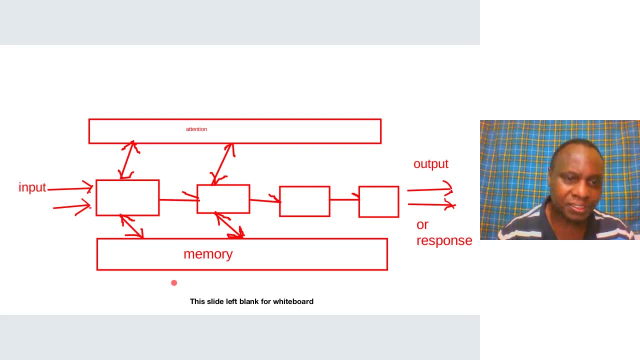 sorry, sorry, i did not share the screen. but anyway, sorry, sorry for that, but i hope the discussion has been clear. uh, sorry for not checking, uh, that you had raised the comment that the screen had not been shared. i don't know what, uh how it happened that i did not do that uh. but anyway, either way, the, at least i 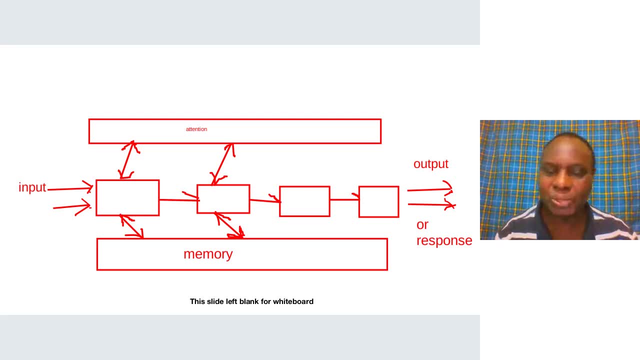 did not share for a long, or i did not present for a long time since that time, um, but most of it was just a text and this time at least open, so i hope that you can see the screen share, okay, well, if i did not share, well, maybe the only thing that i could. 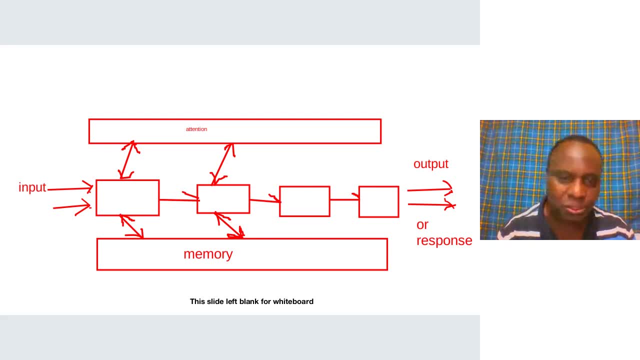 it could cause me to at least display that screen. uh, allow me just a few minutes uh to display, uh the part of the diagram where there was a. i mean there was a diagram, yes, so sorry for that. uh, sorry, i did not check uh to see your comment on the screen share that it had not. 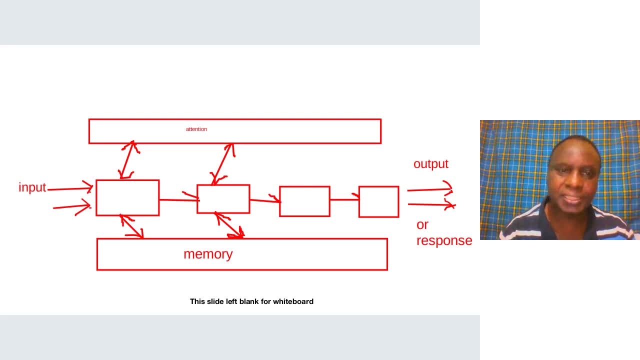 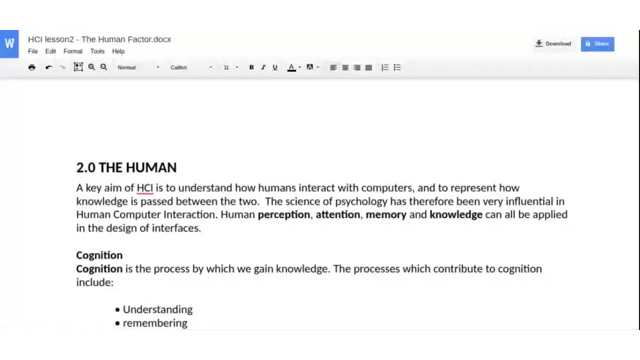 been done. i don't know why. i thought it was a shared. um, i think it would be good. um, i show you the diagram for the that shows a human memory as a multi-store memory as a diagram. uh, so at least let me know. is it sharing? now, how can you see the screen? i don't know, maybe if i forgot to. 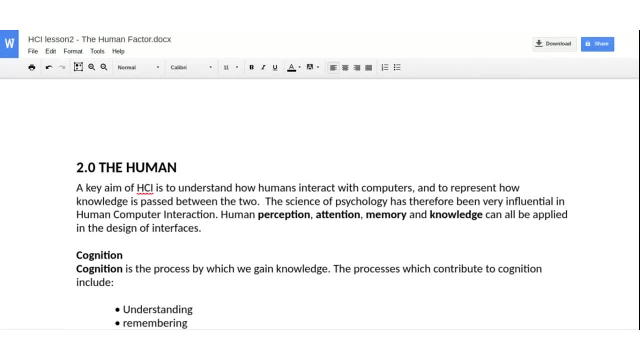 ask us to confirm, please, as you see the diagram now that you already talked about. yes, thank you for uh, winnie, and a brand confirming that now the screen is sharing, and also i want to also appreciate uh, angela, confirming that uh, our, my, the audio has been very, very clear. that's great. thank you so much for those that are confirming. 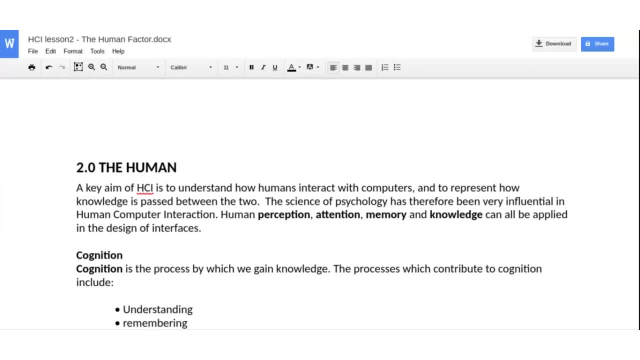 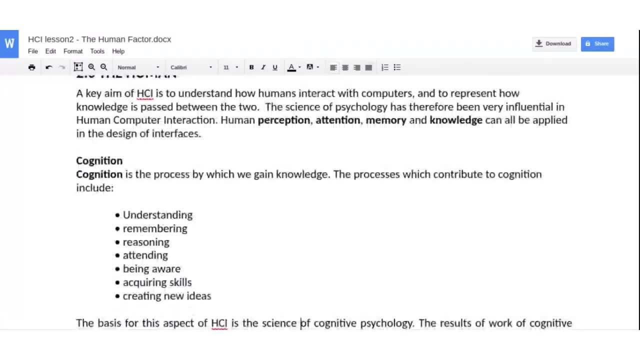 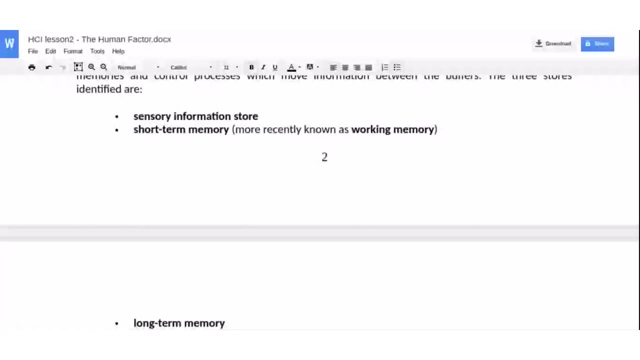 uh, that the screen is sharing now. so what i want is just to display the the image- and, of course, you'll see it later on at your when you access the document- just to show. but there is this document. uh, it's not saying much other than what i've just said. 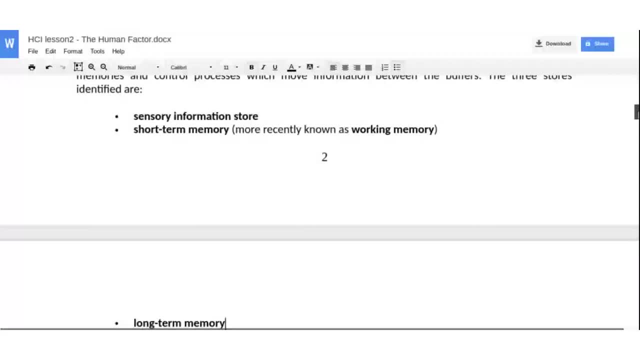 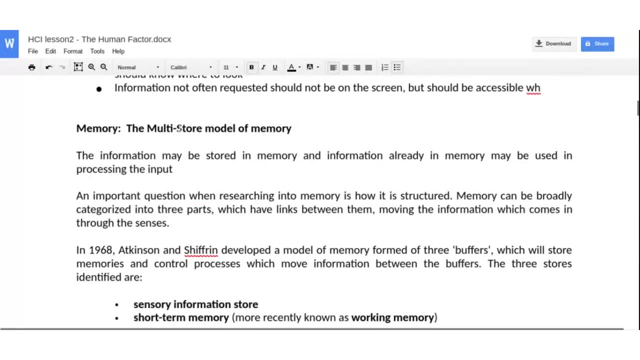 about the, the multi memory model of memory. we call it the multi model of memory. multi model of memory. we see that the memory can be looked at as a comprising of three buffers: the shorter memory, the, or which we also call uh, i don't know. so we have the sensory memory first. 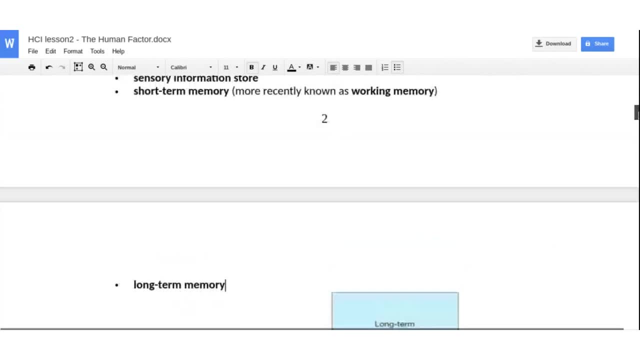 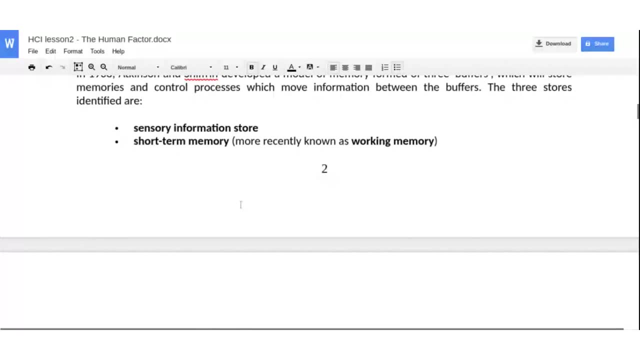 sensory store. you can call it sensory store or sensory memory- and then there's a shorter memory. now this is a now again. uh, for the sake of comparison, because this is almost a coming from the information processing model. but now these are other researchers now trying to look at the. 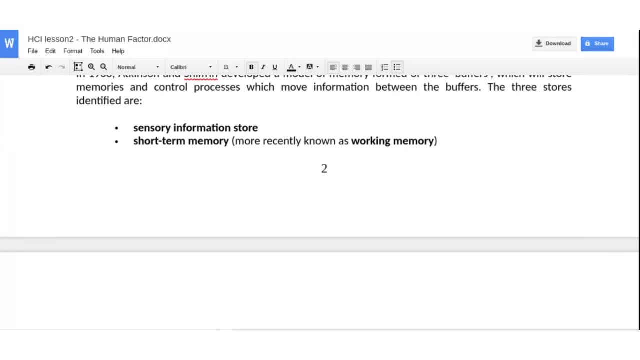 memory and say again, trying to compare uh human memory and the memory of the computer. now you remember that the computer we have the ram, which is uh normally. sometimes you also even call it the work working memories. you see, it is memory that is at work when the computer is working. 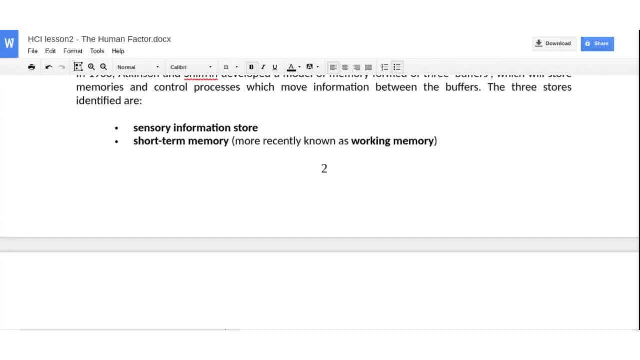 that's where you run your software. when you are accessing a software, you're actually accessing it from the the ram, um, when it is running, uh, and then, of course, when you want to store something permanently, then we put it in there in the secondary memory, and so the comparison is that a 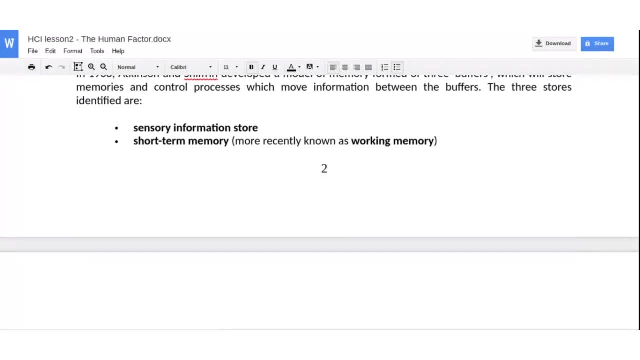 shorter memory compares with the ram and the long-term memory compares with the secondary memory and of course, the, the sensory memory or the sensory store. uh would be more of buffers. so where uh some? and of course these buffers are normally uh at the, the output and input devices. you see sometimes uh uh when you are sending. 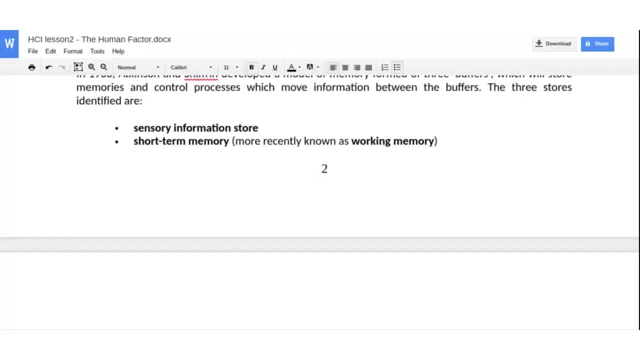 like when, uh, maybe, if something, somebody is able to type very fast, uh that the maybe than they might find that, uh, what they are typing may not reach the the memory immediately sometimes, uh, because that, uh, the content is very fast, but if, if something is not able to get to, yeah, to the memory, you know where it can actually. 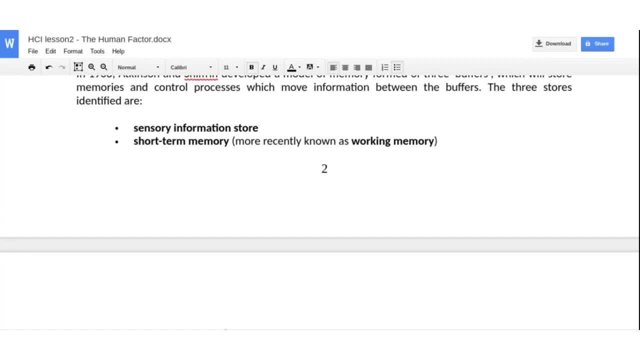 a where the the part which can actually call. now, this is a. it has written memory. maybe it may have to be put at some place. we can call a buffer: uh, when it is not processing, it is put in manner at a buffer and sometimes actually this buffer is actually part of the ram also, but it's a place. 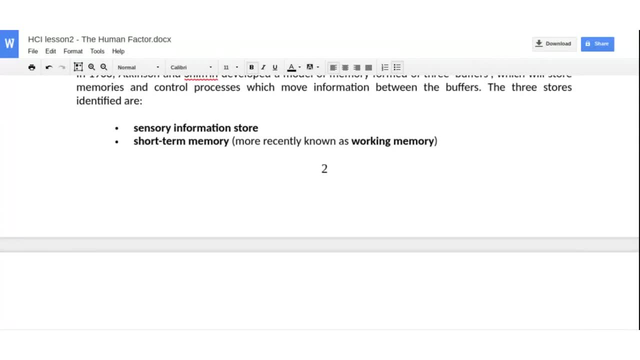 where something is kept before it is, it can reach the processing stage, uh, you know, especially to be processed by the proper area of, uh, uh, the, the ram, and then, finally, if you want to store it permanently, then you have to cause it to go to the secondary memory. so there is that comparison. uh, that is. 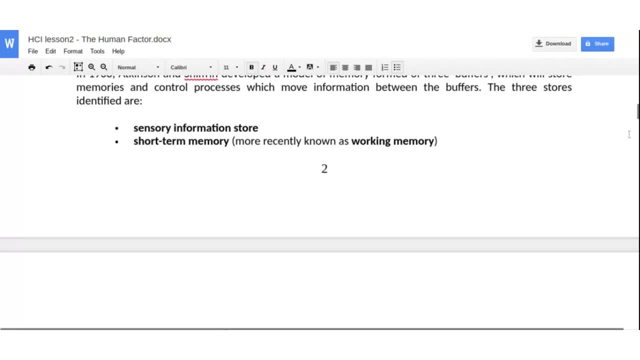 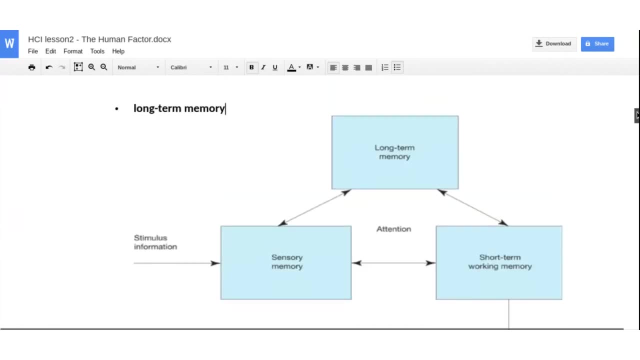 being done here, but otherwise. so the diagram here, uh, and as i said, of course you'll see it, so it's so, this is a diagram that captures the concept and, um, i would do. i will not explain more, i just wanted to just display, now that i realized it had not been displayed, uh, but it's very simple. 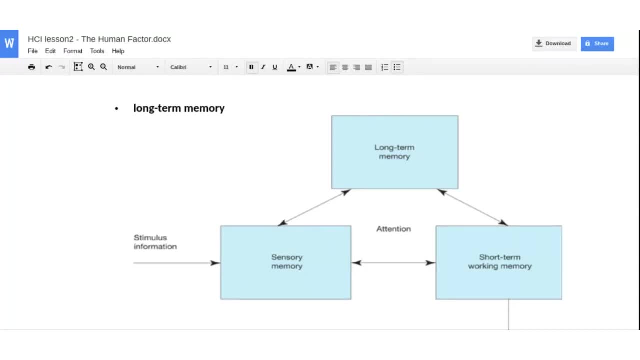 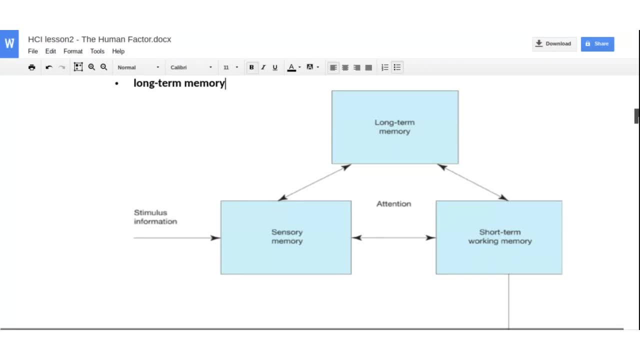 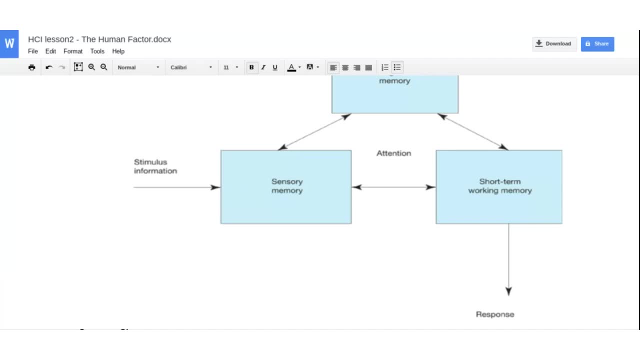 well as the other one which we will not, we are not able to display, but which i drew at the white board uh, which shows: uh the um, the model, the human information, uh processing model, now put into a diagram form. so okay, i think that's enough. i want to remove the screen shell again. 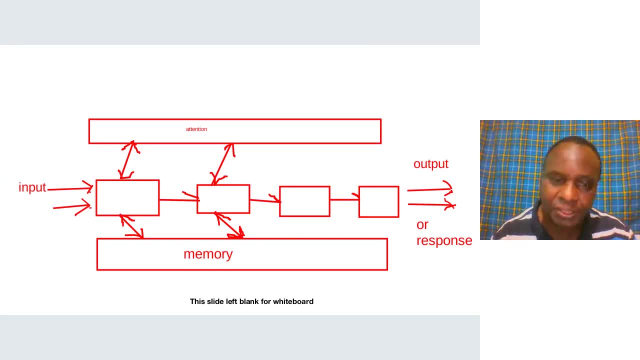 uh, so any question, any comment? uh, in a point of clarification. so just a few minutes. uh, then we should be done with the class. so again, i will allow you to respond to the discussion forum at your own time. you can use it. still a lot of time remaining for this class. 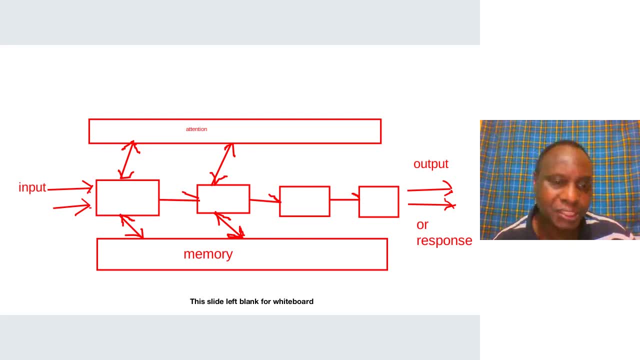 you could use the remaining time to respond to the discussion forum. uh, issue for this particular topical area. uh, this is our topic two. uh, and for for now, the far that we have reached. uh, there is um an issue or is there for discussion, for replying, to respond to at the discussion forum for this? 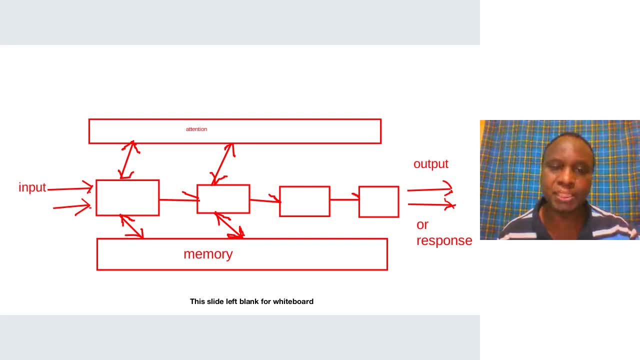 particular. so you go to topic two and you get the discussion forum there. you click that and it takes you to the question or the issue of discussion and at the at the place for that to create a discussion, uh, and it takes you to a discussion forum. so you know your meaningful. 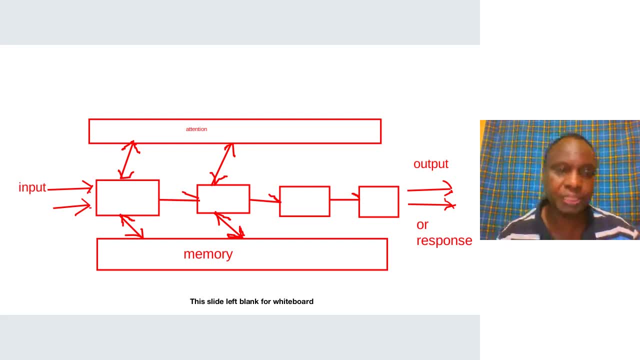 scenes like where you've sat for a while in a different class and the topic of lecture that attendees are more comfortable pod, of course, for that purpose, uh, but just reminding us again, it is very important that you make sure that you have responded to the discussion forum. 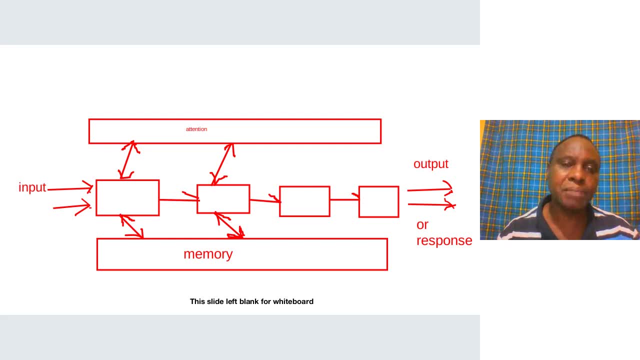 because, uh, it is part of the evaluation. it will certainly account, uh, when you come to evaluate the evaluation for the assignments. so make sure that, uh, you always respond yourpective, as same eclectic, leave a reply at the discussion forum, whether we do it together in class or I. 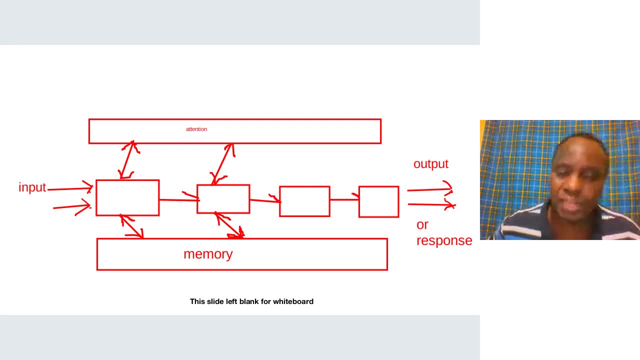 have to ask you, as I'm doing right now, to respond at your own time. we don't want to remain view this time. now. I want to allow you some time to respond to the, to the discussion forum, and but also that you don't, just in case you don't. respond immediately. make sure that you don't take more than a week to respond because at some point it will be blocked- at least after a week to be blocked- and they will not be able to make to leave your reply. so make sure that you reply as soon as possible. 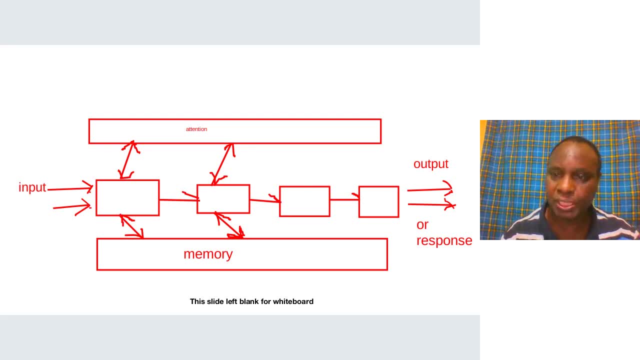 and especially at this time, if I allow, as I closes the session a bit early. then you use the time and respond before you log out. respond to the discussion forum issue. you could do it immediately. the lecturer brings a meeting to a net by coming to the end. 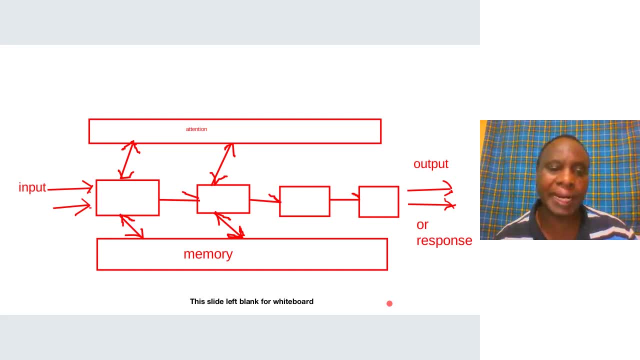 of the class time. all right, so well, i can't see uh any question this far, but maybe somebody want to ask by mike. i think your mic is a is a accessible, so any, if you want to also raise your comment or question by by mike, i think you should be able to also use your mic. 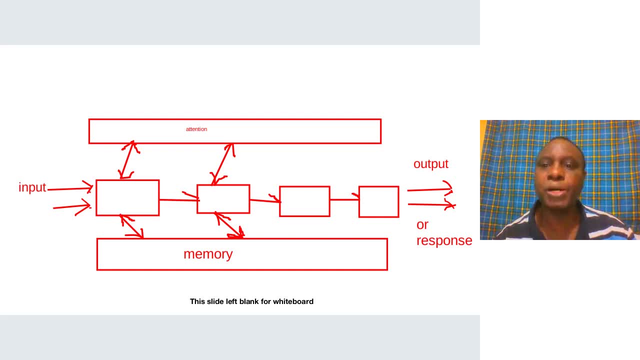 and you are welcome to do that. okay, so, um, giving us a few minutes to make any query before i close our session for today. thank you, bianbo, uh, saying that the presentation went on quite nicely. uh, thank you for that comment, and the dongo is also commenting, uh, about the class. the uh class has been.